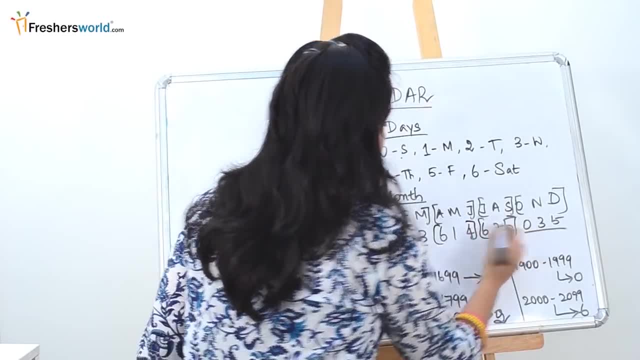 and the middle 2, you can remember it comes in 6, which is 6, 1, 4 and 6, 2, 5.. So first, when you see the answer of sheet, you can write from Jan to December. you can write from Jan to December. 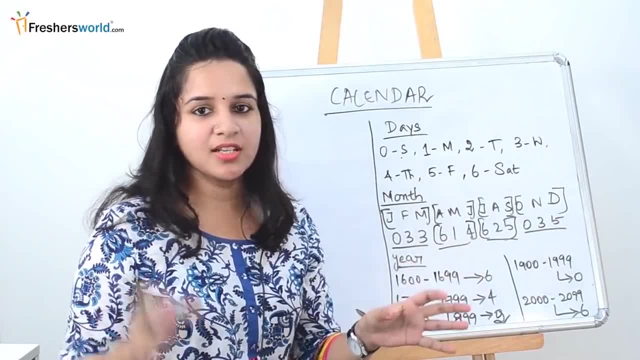 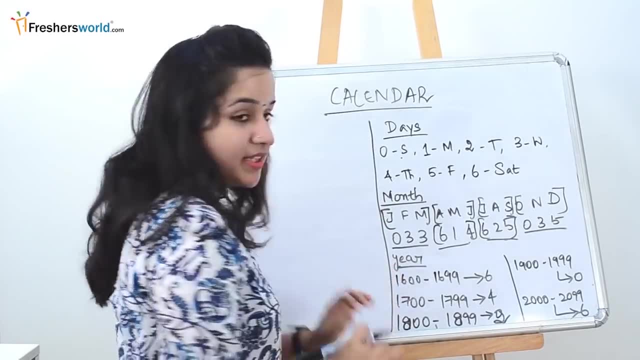 then first fill the first 3 and the last 3 as 0, 3, 3 and 0, 3, 5.. Then in between you can fill it as 6, 1, 4 and 6, 2, 5.. That's how you can remember it as a month, Then for the year. these are the 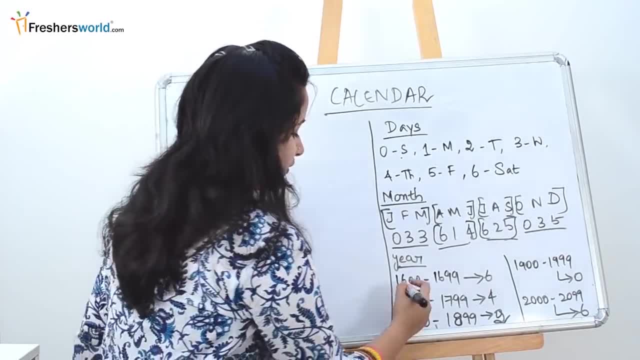 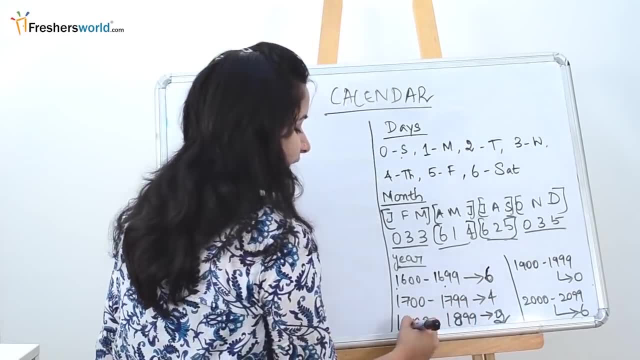 various years that they generally ask in all the type of questions. So from 1600 to 1699, we code it as 6.. From 1700 to 1799, we code it as 4.. 1800 to 1899, code it as 2.. How to remember this Go? 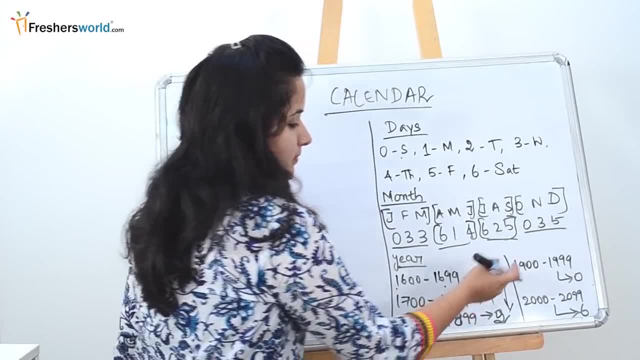 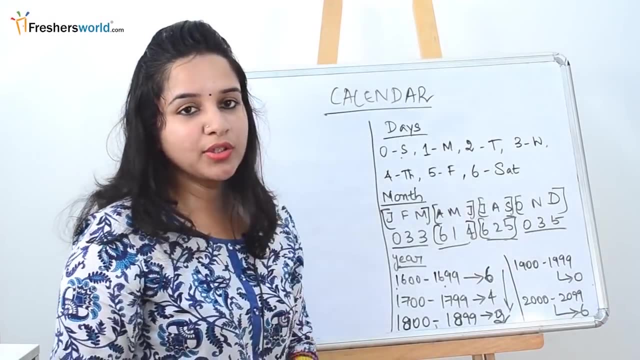 in the descending order from 6,, 4,, 2.. 1900 to 1999, it is 0, and 2000 to 2099, it is 6.. So how do we do it? from days From Sunday, we actually 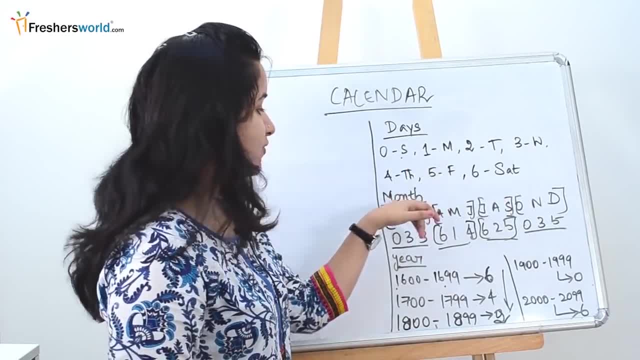 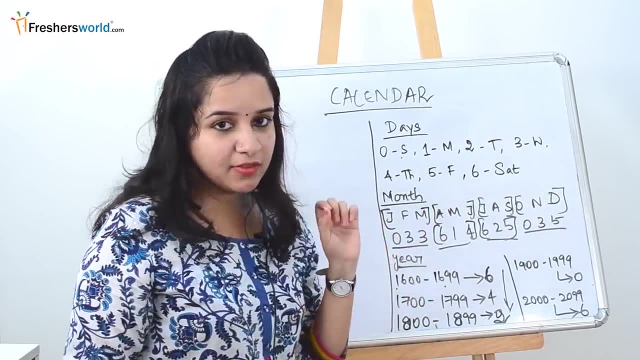 code it till Saturday, So 0 to 6.. Next for month: remember the first 3 and last 3, then fill the middle from Jan to December. Similarly, for year, we are starting from 1600 till 2099.. How do we do? 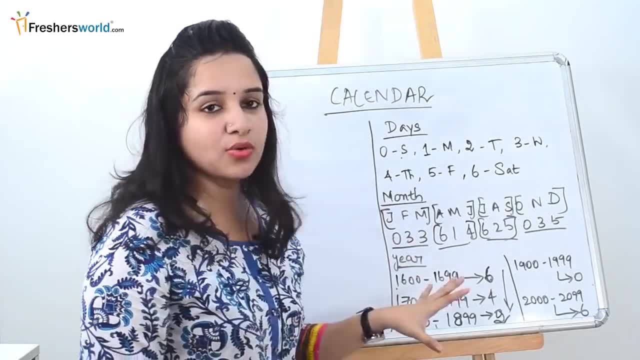 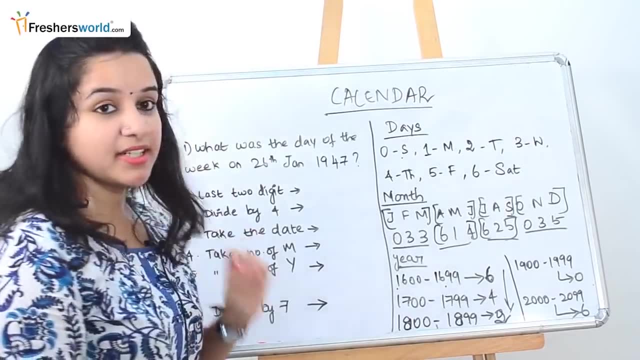 it 6, 4, 2 and 0, 6.. So remember these codes for solving the calendar problem. So let's get started with a simple question. Okay, the first question that they have given is: what was the day of the week on 26th Jan 1947?? So this is the. 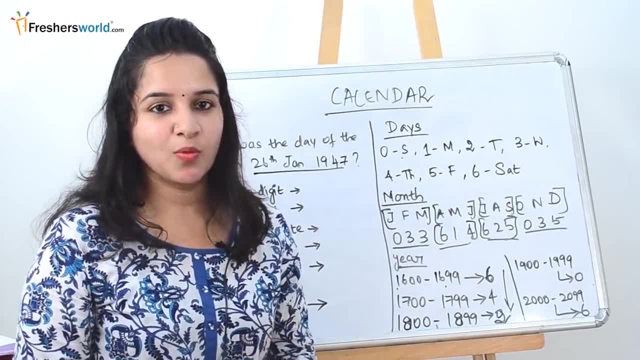 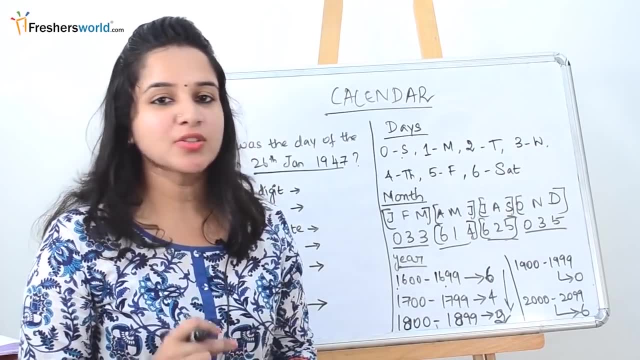 question that they have given. So there are basic 6 steps one need to follow to answer this question. Those are very simple steps. So once you understand the concept of these 6 steps, you can solve it within 15 seconds. So 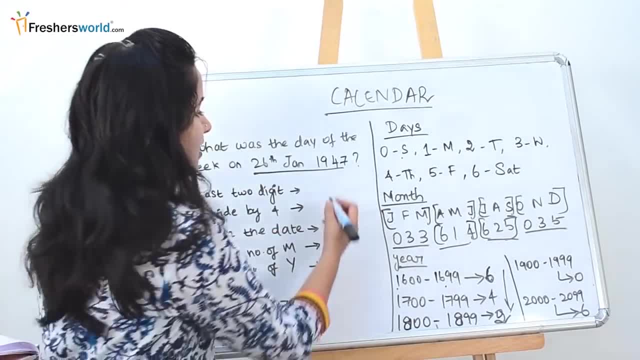 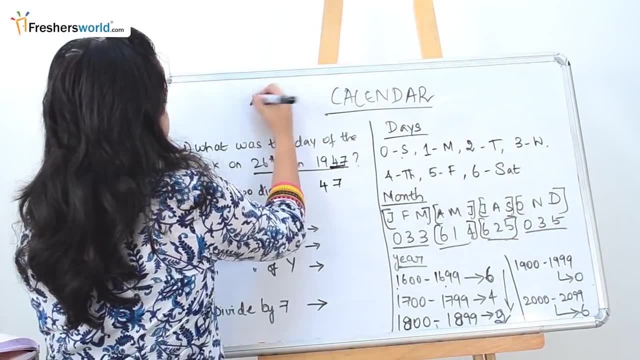 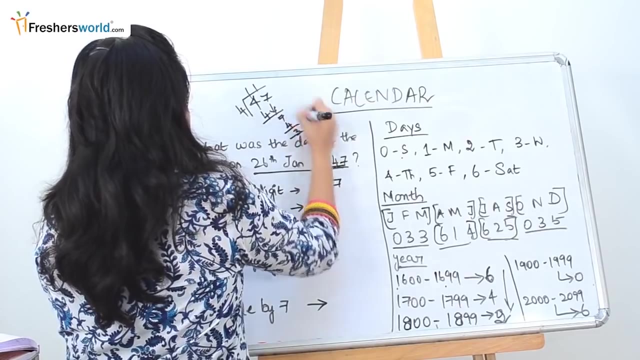 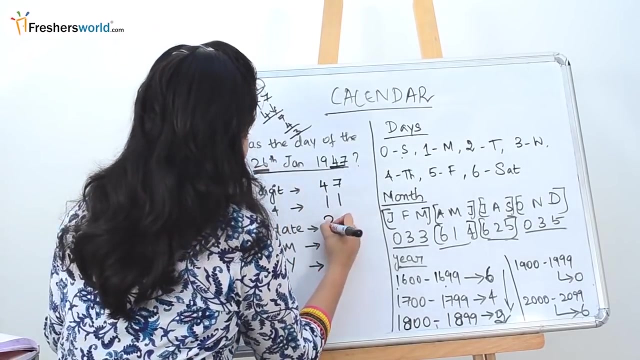 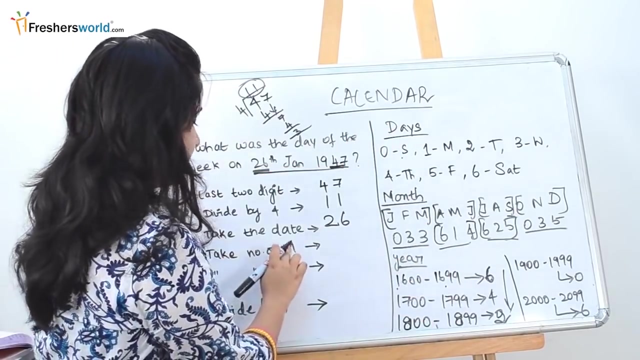 first you have to take the last 2 digit of the year. So what is the last 2 digit of the year? 47. So next divide it by 4.. So take your quotient. Next take the date. So date is nothing but 26th. Next take the number of the month. So from here these things will come into place. So what is the number of the month? What is the month? Jan? So Jan is nothing but 0. So we take 0 here. Next take the number of the year. So from here these things will come into place. So what is the number of the month? What is the month? Jan? So Jan is nothing but 0. So we take 0 here. Next take the number of the year, So from here these things will come into place. So what is the number of the month? What is the month? Jan? So Jan is nothing but 0. So we take 0 here. Next take the number of the year. So from here these things will come into place. So what is the number of the month? What is the month? Jan? So Jan is nothing but. 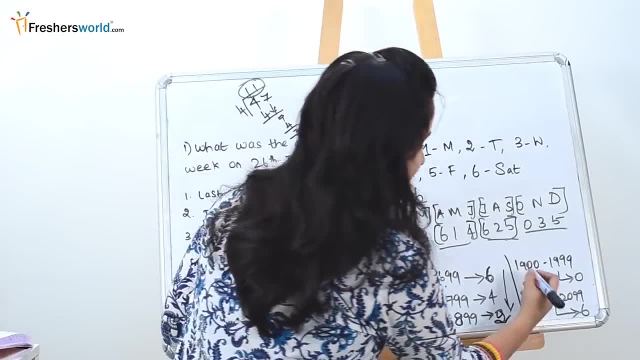 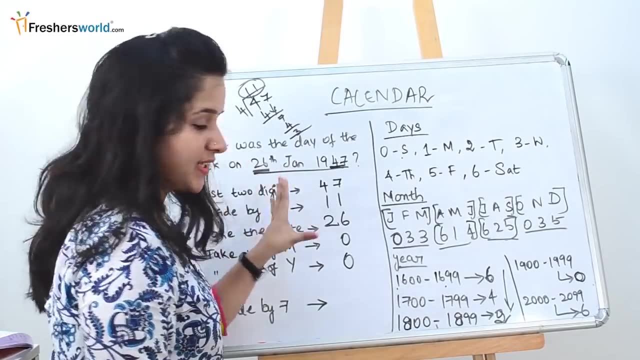 so year is nothing but 1947, so 1900 to 1999, which is also zero here. so we take it as zero. so now you add these first five steps: 7 plus 1, 8, 8 plus 4, 8 plus 6. 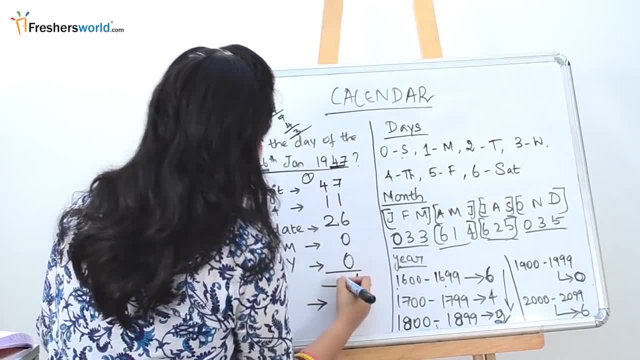 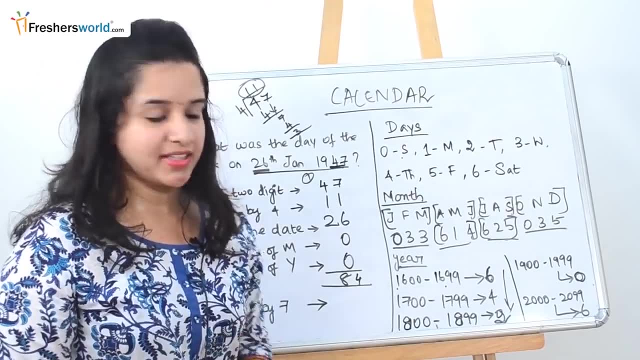 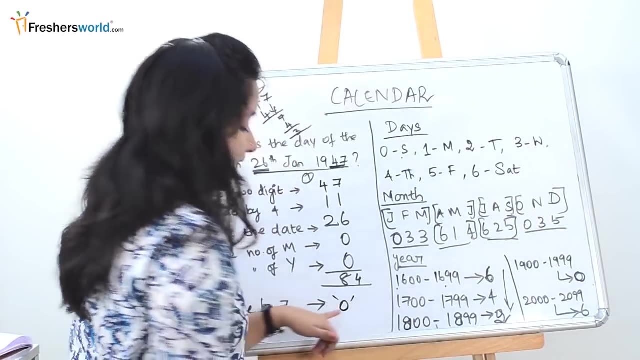 is 41, 5, 8, 84, so your total is 84. what is the question? what was the day of the week? so how many days in a week? seven days. so you're dividing 84 by 7, we know that 12 sevens are 84, so you will obviously get the reminder as zero. so 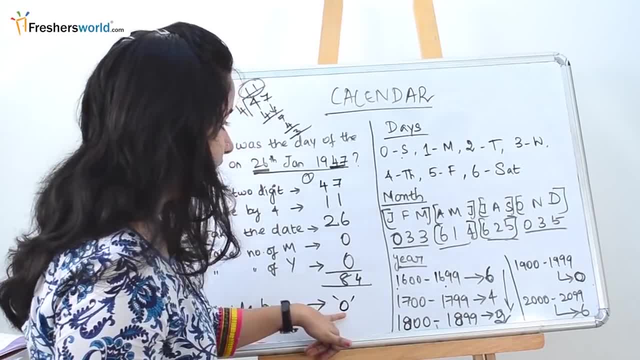 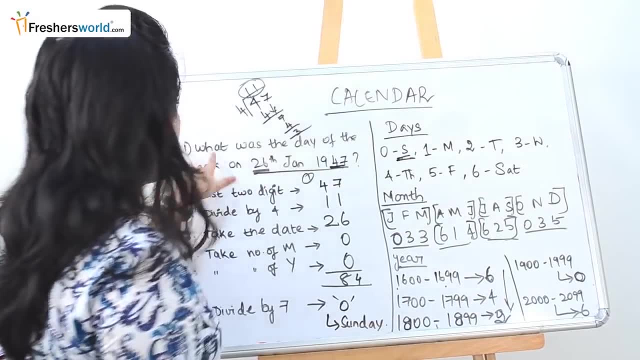 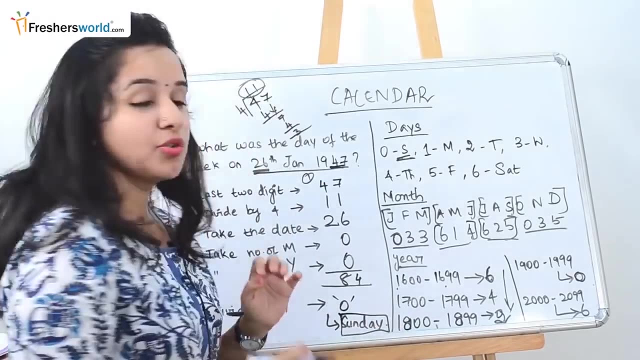 you have to take reminder here. so zero. so what is it corresponding to? zero is nothing but Sunday here. so what was the day of the week on 26th Jan 1947 is nothing but Sunday. so in this question, what you need to know for the first five, 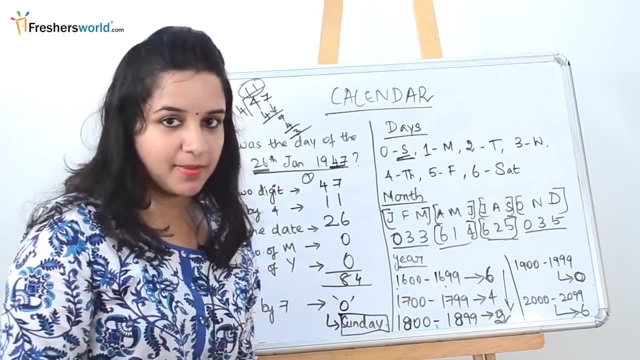 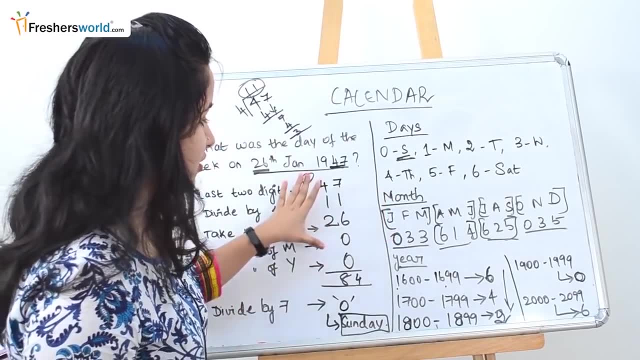 steps. first, you have to take the first two digits divided by four. you have to take the first two digits divided by four. next, you have to take the date. next, you have to take the number corresponding to month, number corresponding to your. once you get the first five, add it, then they: 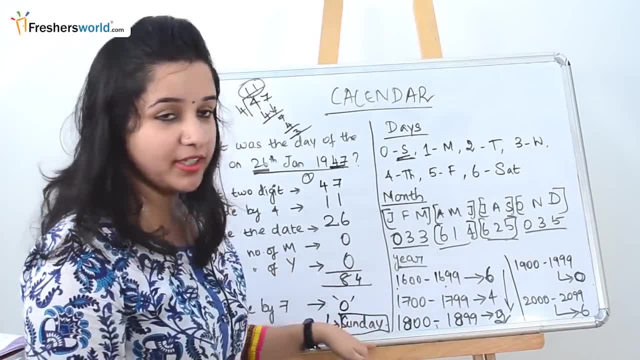 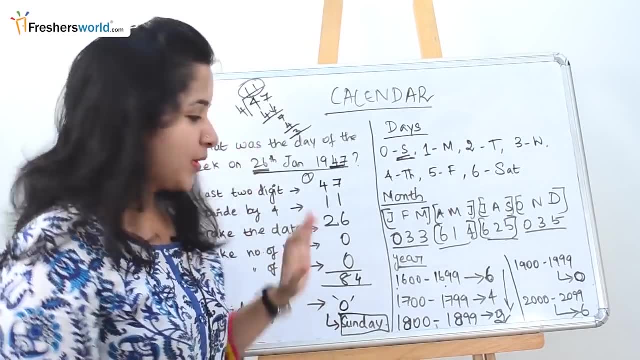 are asking for the day. so you will divide it by seven. the reminder of it nothing but corresponds to the number code of the days, so you can directly write it. so initially it will be really tough, but once you understand the six steps really easily you can finish off the sum. let's solve another example. so 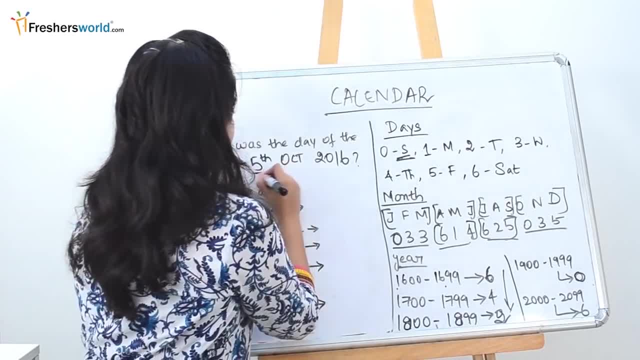 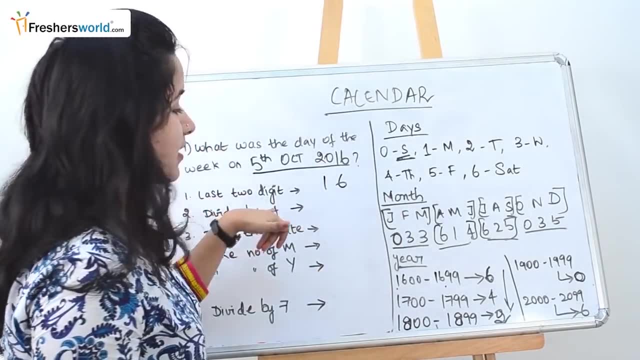 the next question is: what was the day of the week for 5th October 2006, 2016? so what is the first thing you have to do? take the last digit, which is nothing but 16, so dividing it by four, you know the quotient will be four. next, 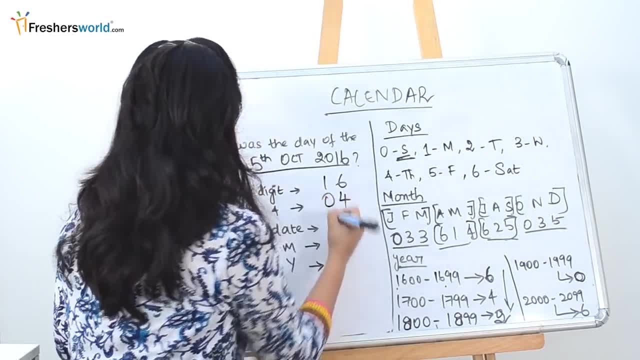 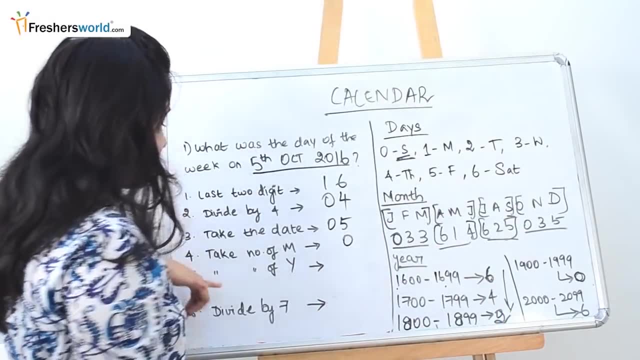 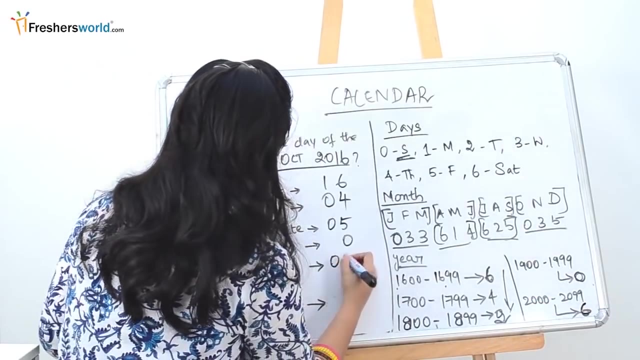 take the date. date is nothing but fifth. next, take the number of the month, so October. so what is October? October is again zero here. so take the number of the year, so year is 2016. so 2000 to 2099 is 6. so we are taking six here, so add all of these. 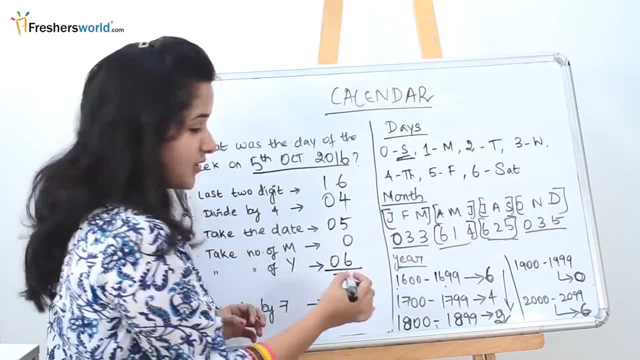 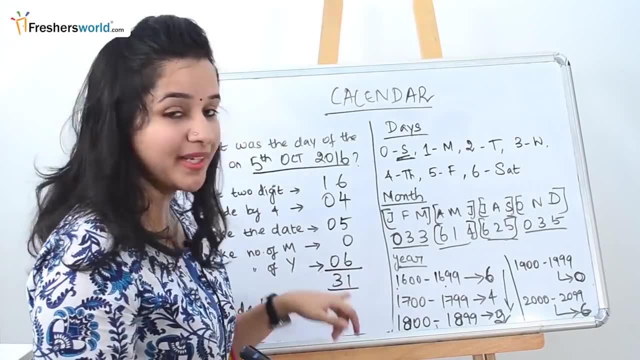 five. so if you add all these first five steps, you will get the value as 31. so what do we do? they were asked the question the day of the week, so we divided this 31 by 7. so let's divide 31 by 7. you know 7, 4, so 28 and the reminder. 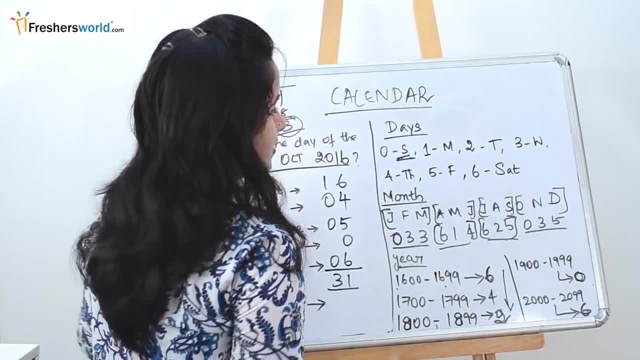 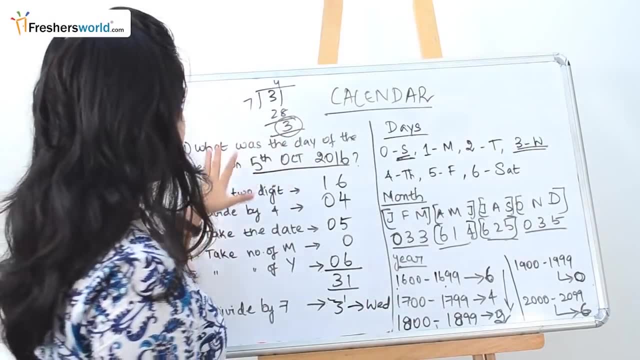 is 3, so we take the reminder here. so code number 3, so 3 falls under Wednesday, so the Wednesday. so what is the day of the week on 5th October 2016 is nothing but Wednesday. so what was the day of the week on 5th October 2016? is nothing but Wednesday. 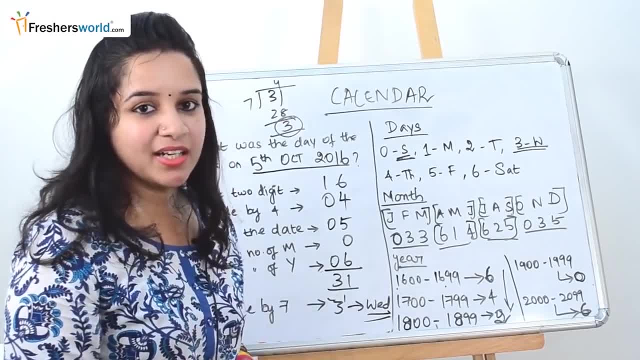 so what is the day of the week on 5th October 2016 is nothing but Wednesday but Wednesday. so we now we can see that how easily we solve this sum. so once you practice three, four sums on the same topic, then easily, within seconds, you can. 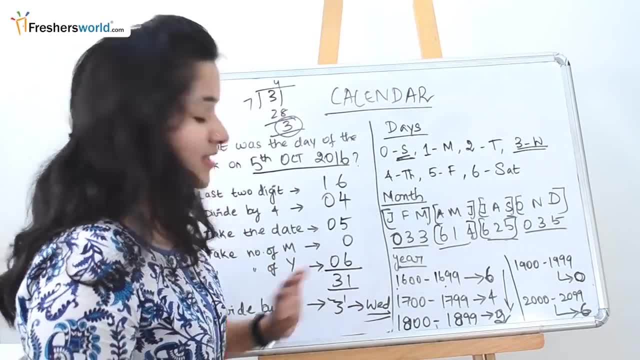 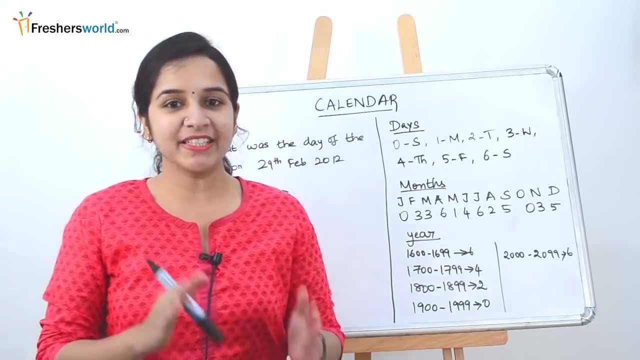 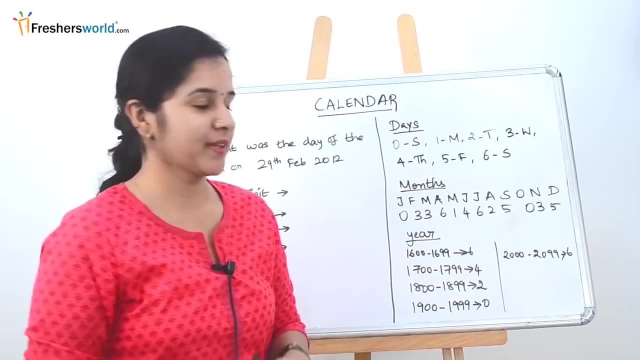 do it. you know the steps. you will just substitute the value. you can easily find a value for it. the first part of the calendar problems: we found how to find the day for normal year. now in this type, we are going to first start discussing about how to find the day for a leap year. so how did we do it? the first step: 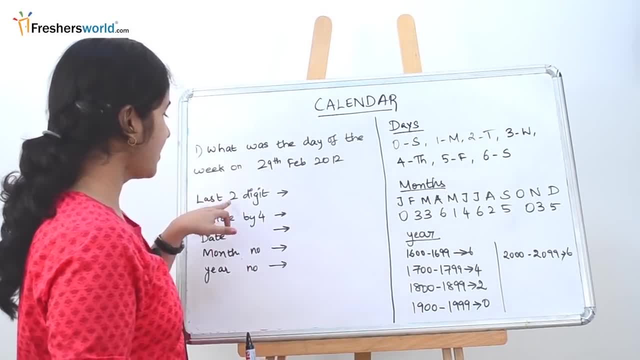 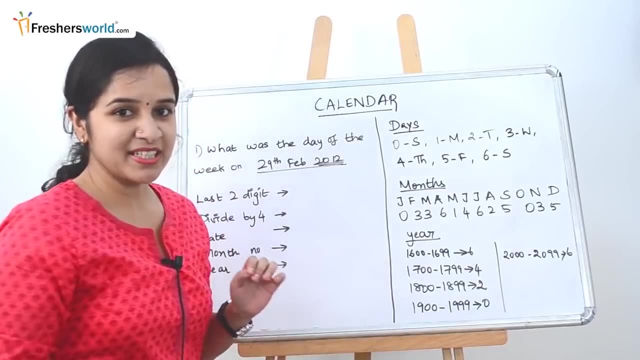 as usual, we have the first five steps, so first we have to take the last two digits. so the question that they've asked is: what was the day of the week on 29th- 5th 2012, which is obviously a leap year? last two digits of the year, so which? 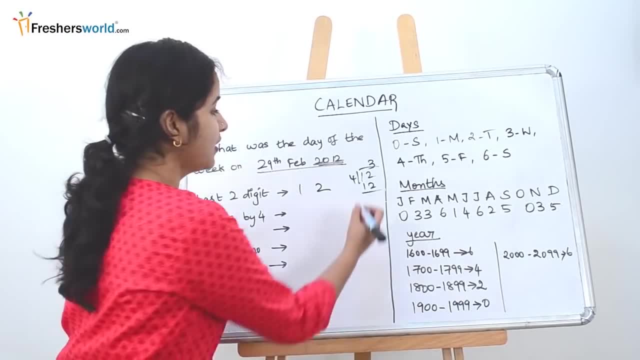 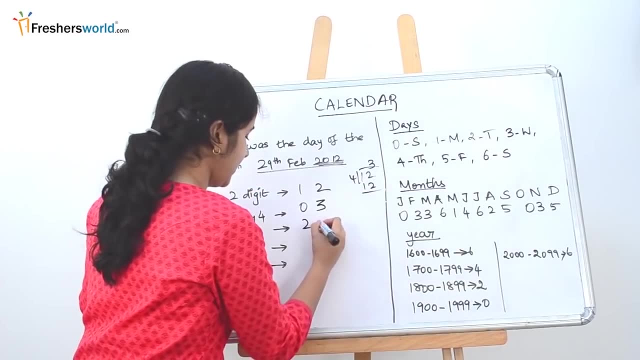 is 12. next step is divided by 4. so if we divide 12 by 4, we know that the answer is quotient is 3, so we put it here. next is the date. so what is the day that they have given 29? the next is a month number. so February corresponds to 3, so we put: 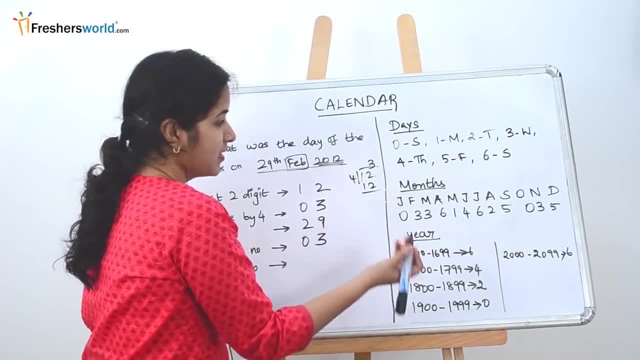 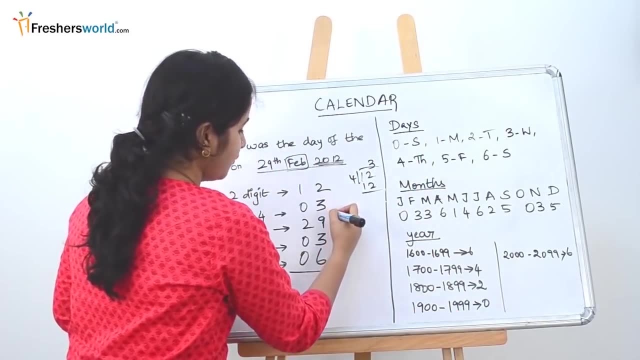 3, so we put 3. so next is the month number, so February corresponds to 3, so we put 3 here. next is the year number, which is 2012. so 2012 falls between the bucket of 2000 to 2099, which is nothing but 6. now add all these 3 plus 2, 5, 14, 17, 23, so 5. 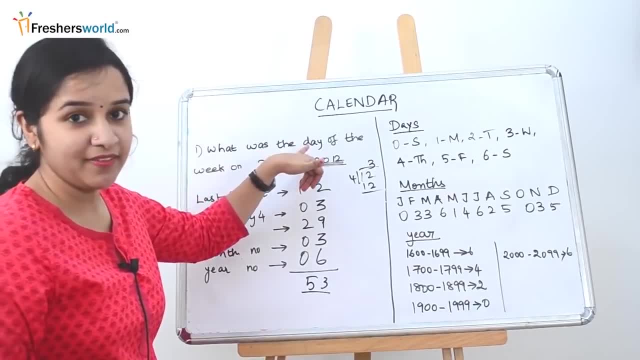 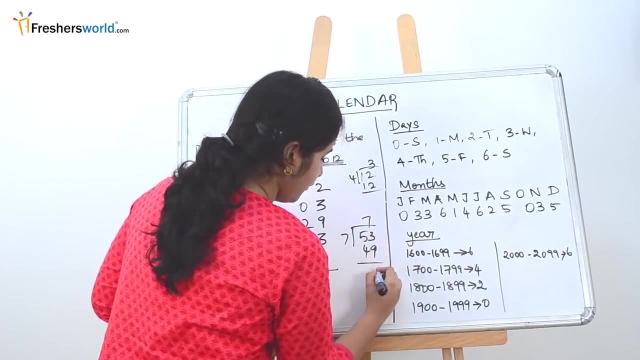 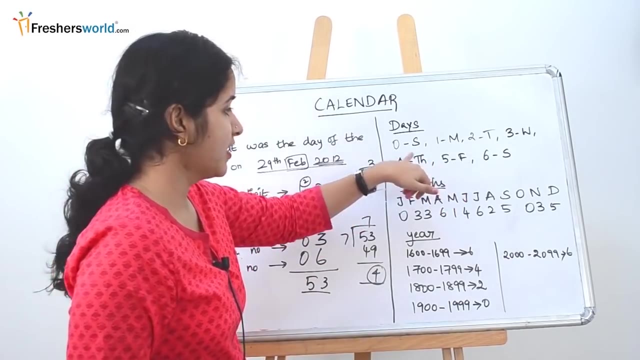 53. so what is the last step? as we know they've asked for the day? we divide 53 by 7, 7, 7, so 49, so 4. so generally for a normal year, what do we do it? we take 4 and we find the corresponding number for that. so 4 is nothing but Thursday. we. 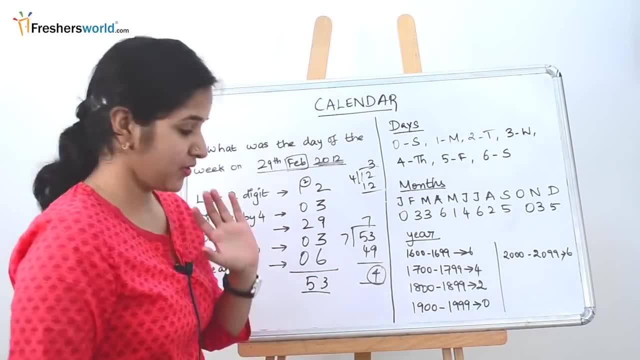 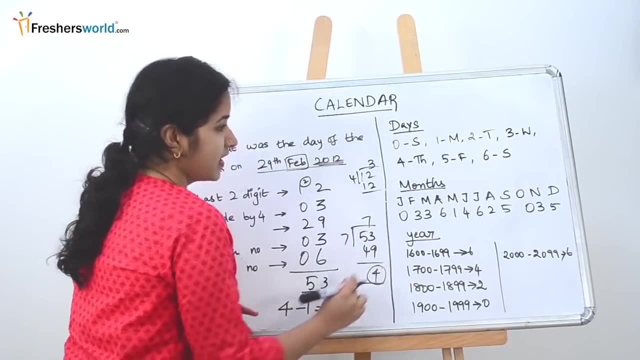 write it as Thursday. but here the catch is, they've asked for a leap year. so what do you do? the same step we are going to do. take 4 subtracted by 1, which is nothing but 3, so 3 corresponds to nothing but Wednesday, so 29th Feb 2012. 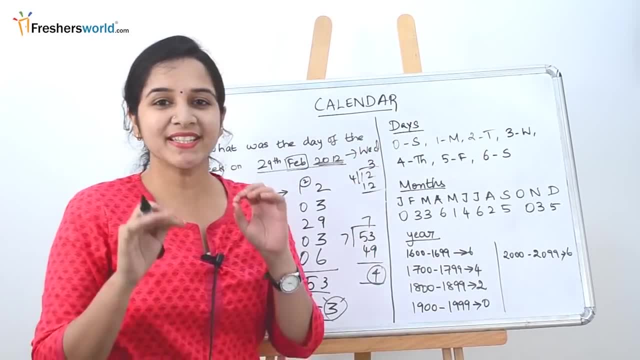 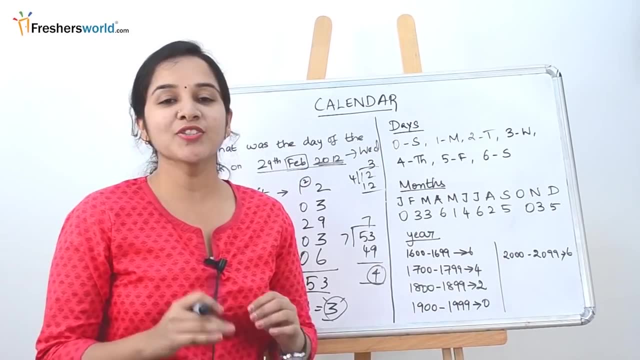 falls on a Wednesday. so it is the same step that we have followed for a normal year. only minor change in the last step is that we are going to subtract it by 1. you can use the same method for any other leap year to find what day it. 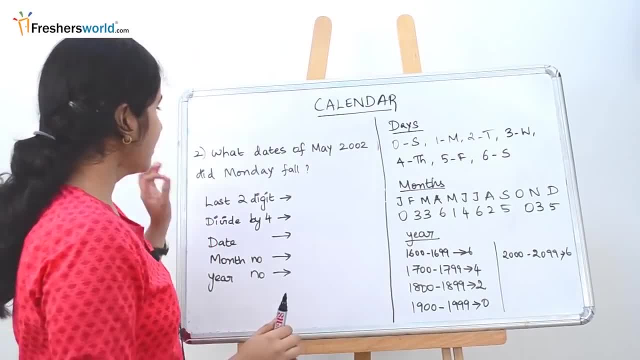 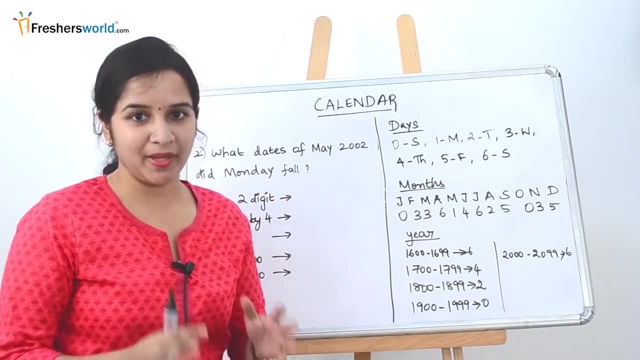 falls on. let's solve some other problems. so the second sum is that: what dates of May 2002 did Monday fall? so what does this question mean? they are asking that in 2002, May, what are the various dates in which Monday has formed? so first, how? 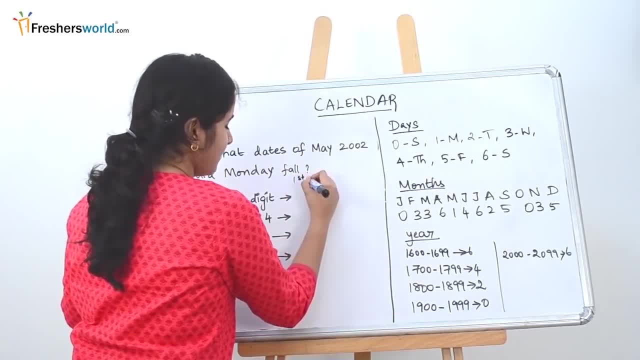 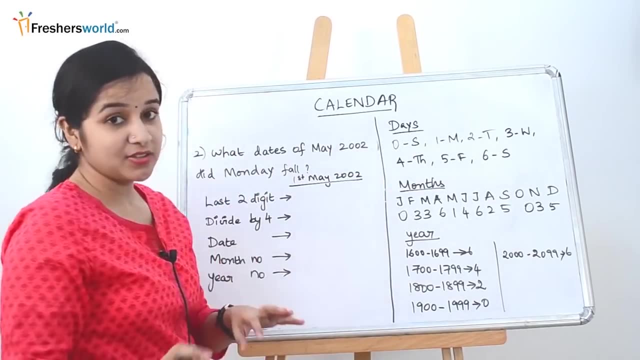 to solve it. the first step is that let's take- we are going to take- the date first, May 2002. we are going to solve it in the usual method that we do the last two digit of the year: 0, 2 divided by 4. if we divide it by 4, we know. 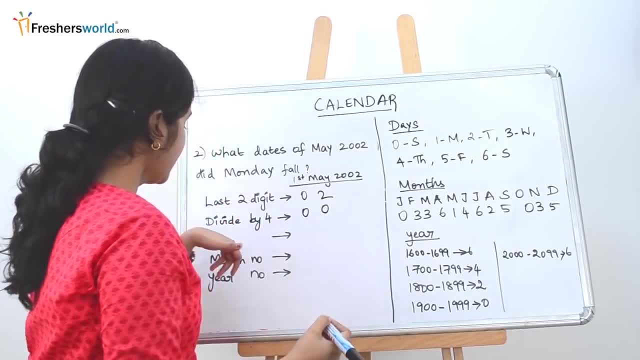 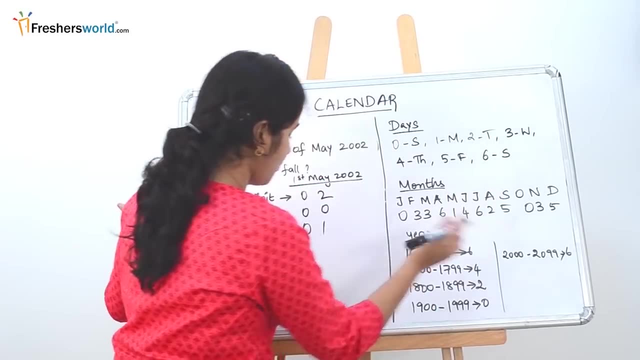 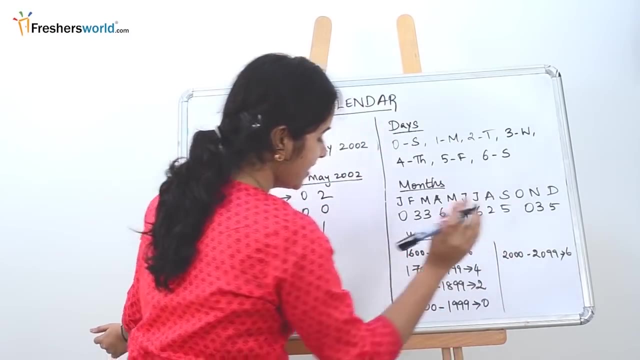 obviously the quotient is going to be 0, next is the date. date is first 0, 1, next is a month number, so it's May. so May corresponds to 1, so you write 1 year number. it falls 2002, 2002 falls under 2000 and 2099, so the number. 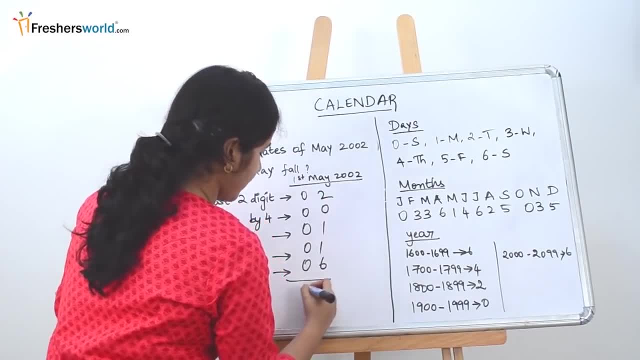 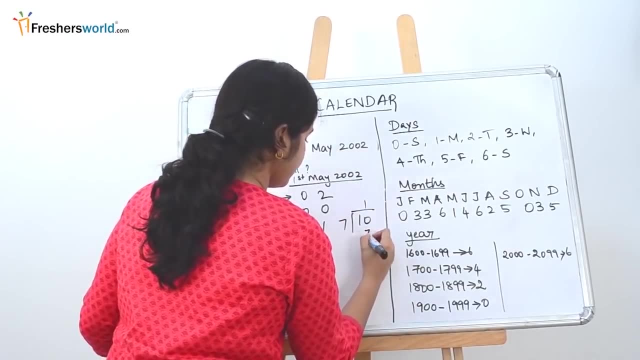 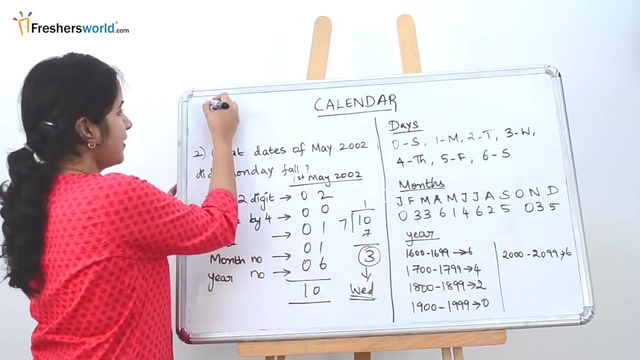 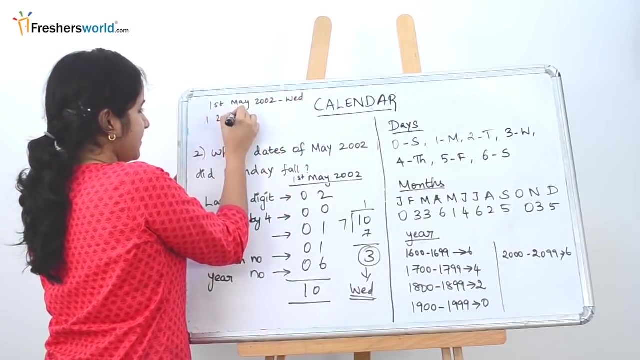 corresponding to it is 6, so 2 plus 3, 4, 10. so what do we do? similarly, we have to divide it by 7, so reminder is 3, so 3 is nothing. but we know it's Wednesday, so first May, first May 2002 falls on a Wednesday. so first, second, third, fourth. 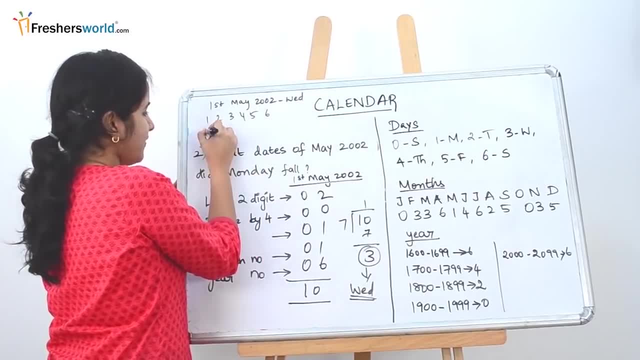 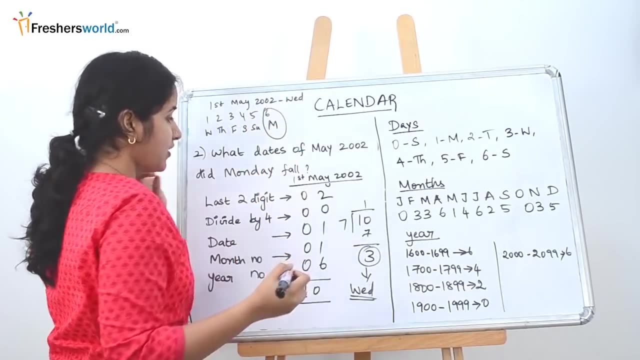 fifth, six, for example. so first falls on a Wednesday, 2 is on Thursday, 3 is on Friday, Saturday, Sunday and 6th is on Monday. so the question they are asked for is Monday. so the first Monday falls on for May is on 6th, so we know. 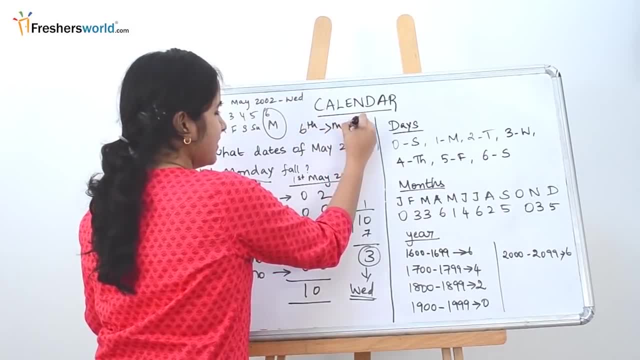 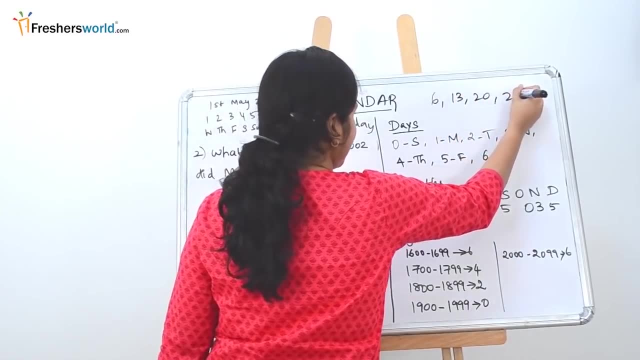 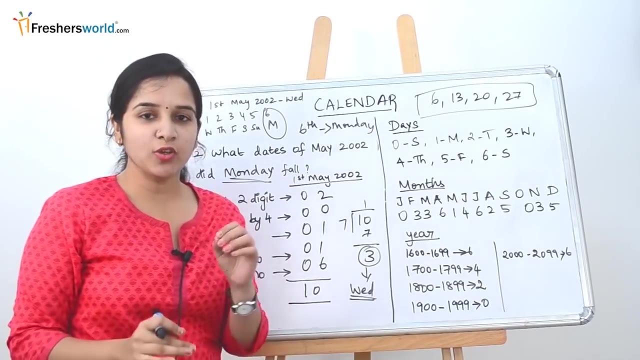 that 6th is definitely a Monday. how to find the other days? it's very simple: you have to just add 7 to it. so 6, 13, 20th, 27. so these are the various dates that will fall on Monday on May 2002. so how do they give the options? 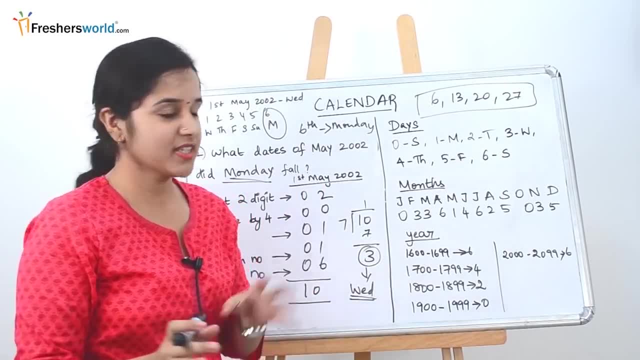 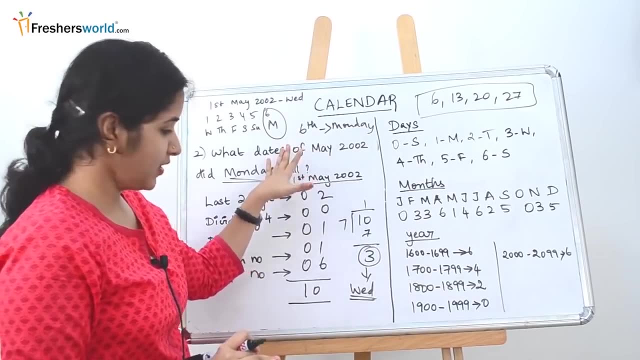 here. they will give you four different dates for in all the four options and they will ask you to find the correct one. do this first. take the first of some month, whatever the month that they have given you. follow the usual procedure. then just put the seven days of the week and then goes to the pertaining to the 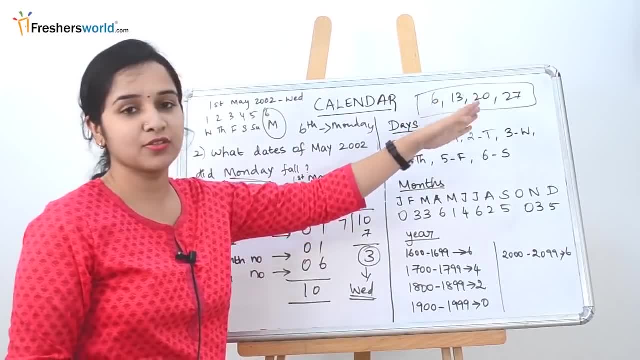 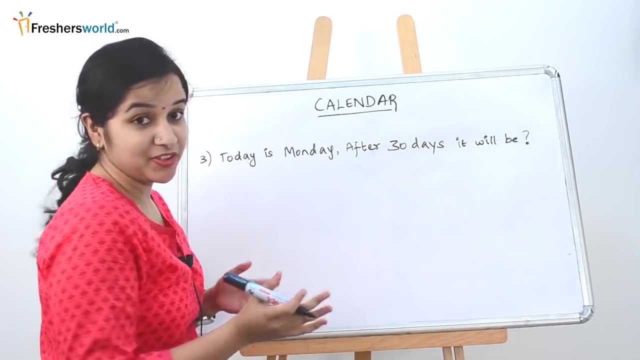 day that they have asked. then you can add just seven to it and find the rest of the other days. this is how you have to do this sum. let's solve another sum. so the next sum is a very simple sum. so what? what is the question? today is monday, after 30 days, what day it will be? so it's very simple. 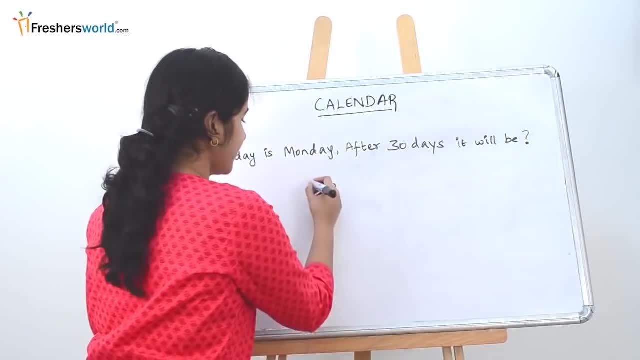 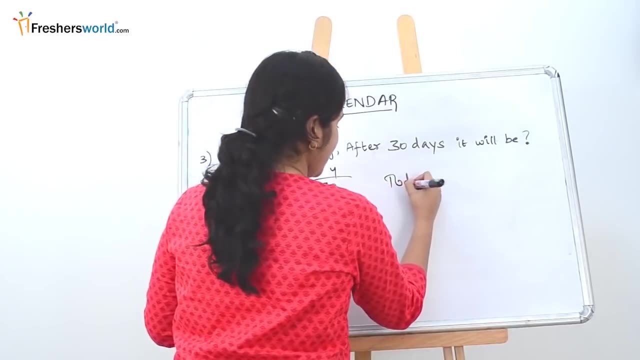 that they are given 30 days. you know how to find a day, it's nothing but divided by 7, 7, 4 or 28, so 2, so the remainder is 2, so today, let's. today is monday, so i add plus 2. 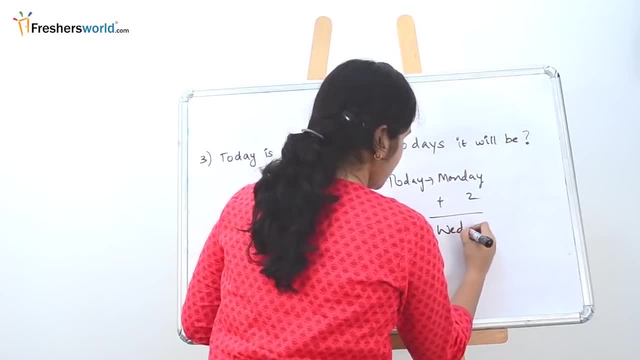 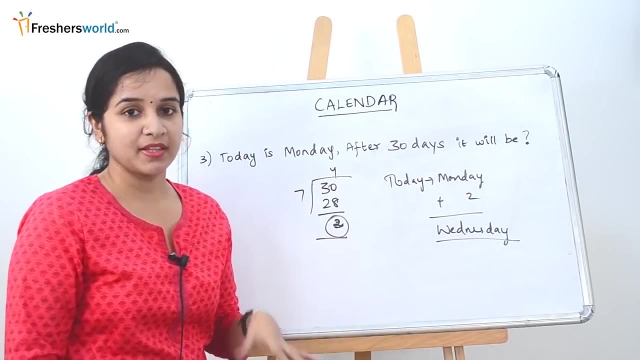 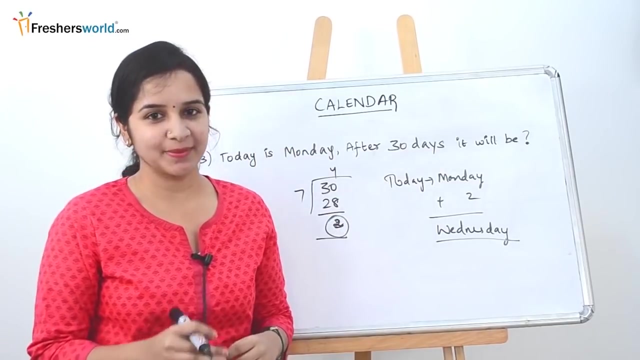 so the next day is tuesday, then it's wednesday, so after 30 days it will be wednesday. this is how you have to solve this sum. they will ask the same question with different days. it will be the same method the will be following. for every other sum, Let's solve another sum. So the next question is: 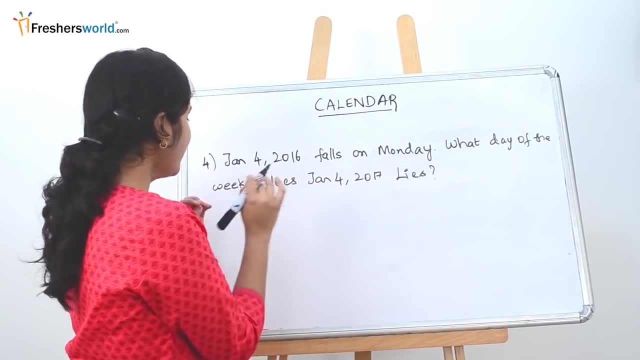 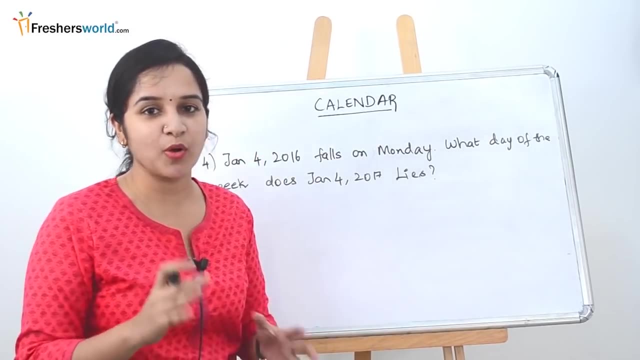 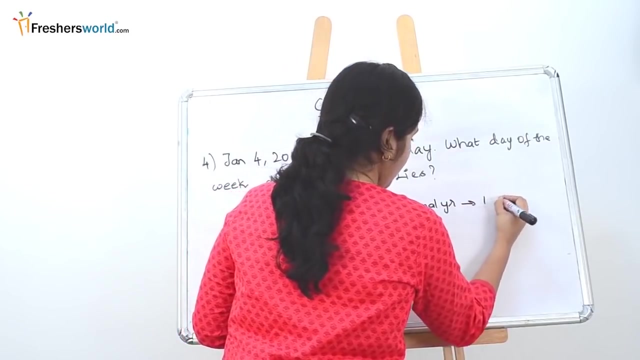 Jan 4, 2016 falls on a Monday, So what day of the week this Jan 4, 2017 lies? So if you have seen our calendar first part video, it would have been discussed about the odd days in a normal year and a leap year. So in a normal year we have one odd day In. 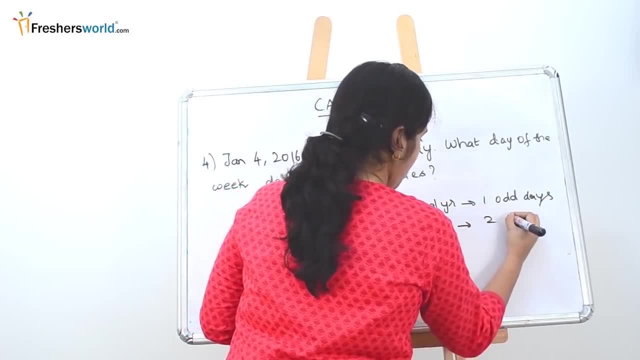 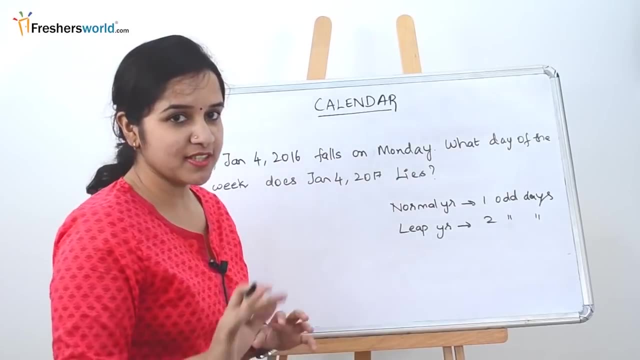 a leap year, we have two odd days, So this is going to be the basic for solving this sum. So what they have given So Jan 4, 2016.. You know, 2016 is a leap year, So it. falls on a Monday, So Jan 4, 2016 falls on a Monday, So Feb will be falling on 2016, where you will have an extra two days because it is a leap year, So it will be plus two. 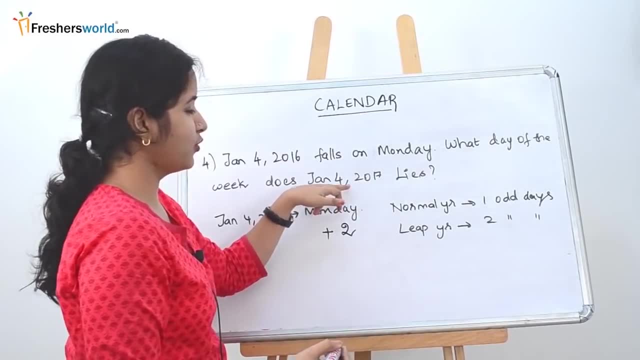 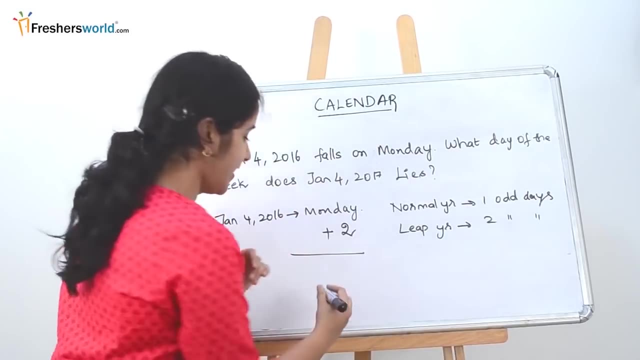 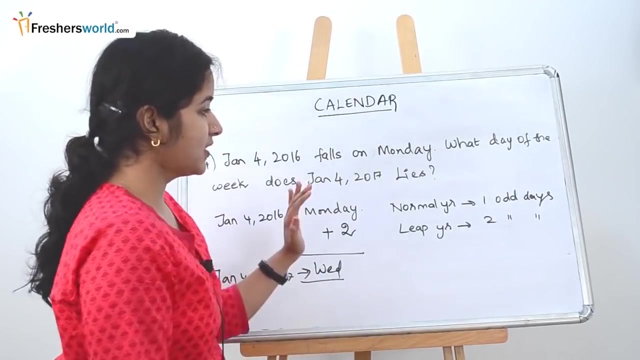 here. So obviously the Jan 4, 2017 following that year will definitely fall on Monday plus two, which is nothing but Tuesday, then Wednesday. So Jan 4, 2017 will fall on a Wednesday. So this is because we took as a leap year. Let's take a normal year. What do you do with it? The same day will take it and you will do plus one. So if it is a Monday, then it will fall the next year on Tuesday. If it is a Thursday, then it will fall on a Friday. So this is the difference. 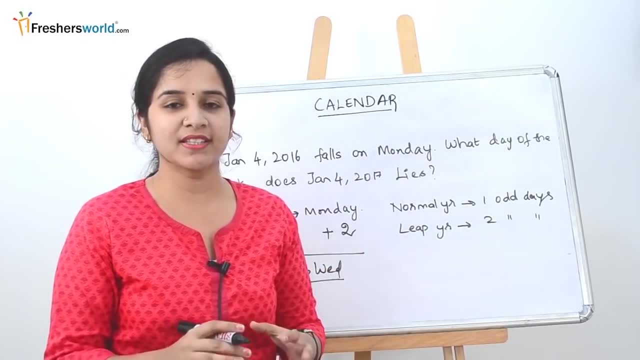 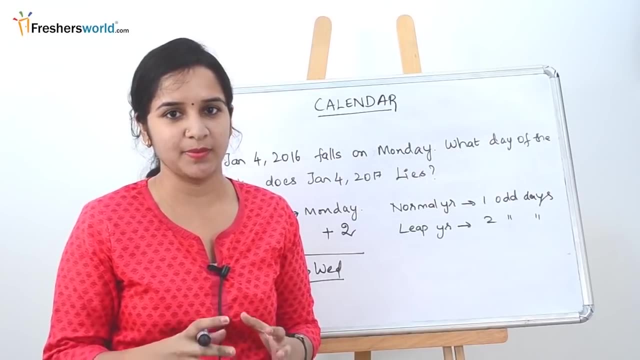 between the normal year and the leap year. So in this video we discussed about how to solve leap year sums and as well as the other basic sums that you might find in a calendar problem. The topic that we are going to look today is calendar part 3.. So the 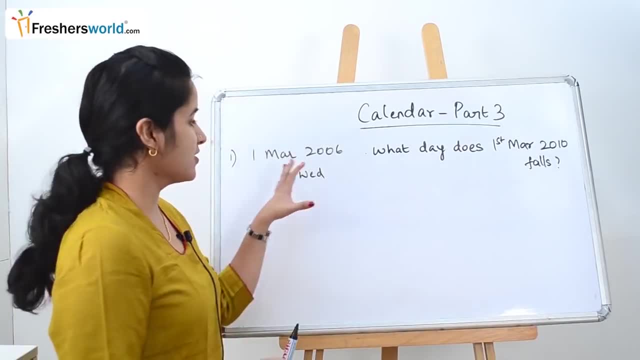 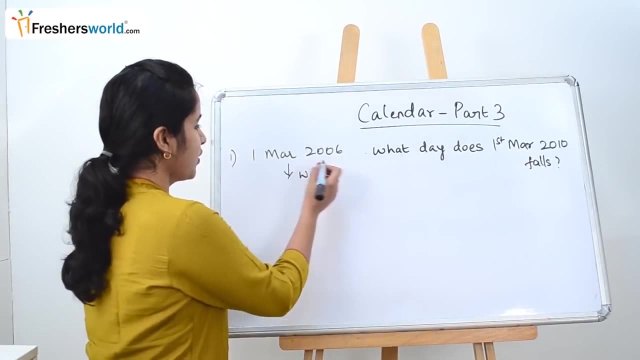 first question is: 1st March 2006 falls on a Wednesday. What does 1st March 2010 falls on? So this is the question they have asked, So how to solve this? So we know that it. 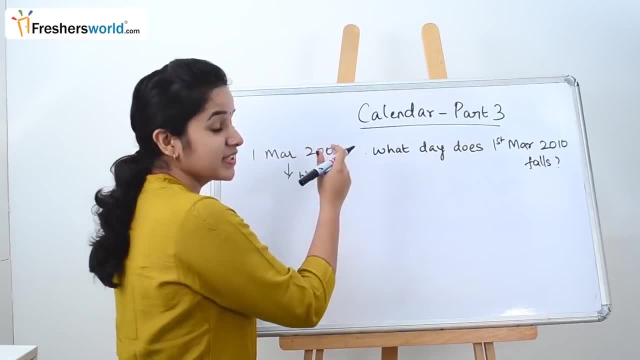 is 1st March 2006.. So it has crossed Feb. So we will start counting it from 2016.. So we will start counting it from 2007.. So 2007 is not a leap year, So it will have one odd. 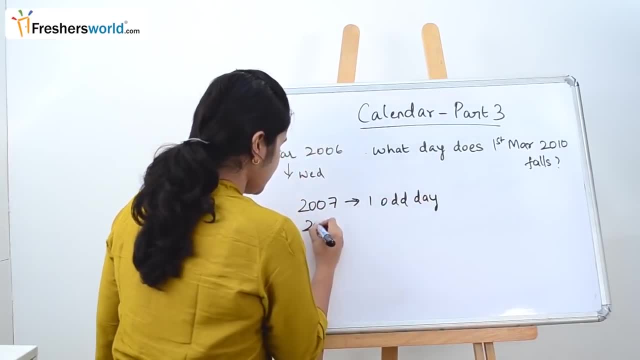 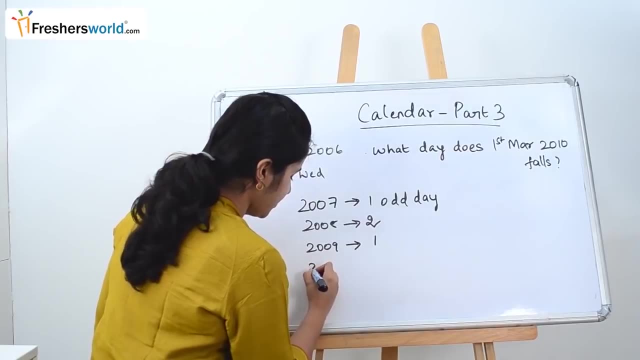 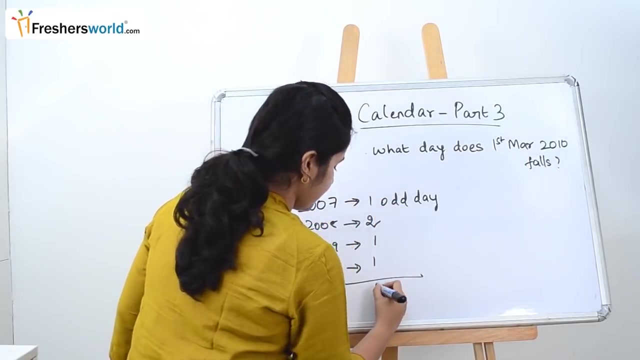 day. So 2008 is a leap year, So it has 2.. 2009 is not a leap year, So it has one odd day. 2010, it has one odd day, So they have asked till 2010.. So 3, 5.. So 5 odd days. 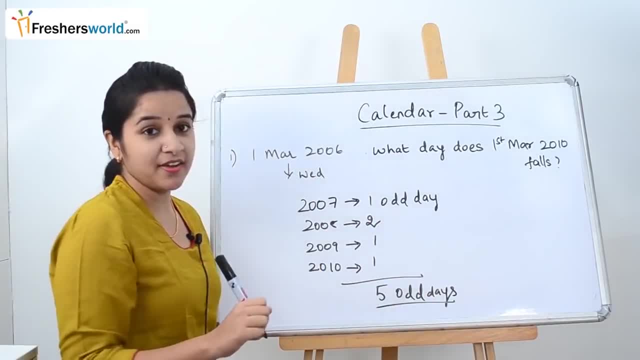 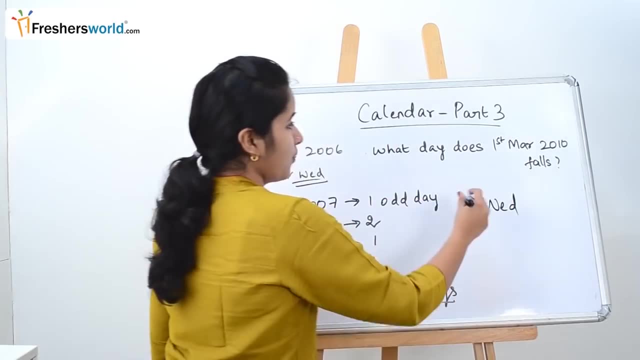 are there, So what do we do? The question they have asked, 1st March 2006, is the day of Wednesday, So the question they have given is Wednesday. So when is 2010,? 1st March falls. 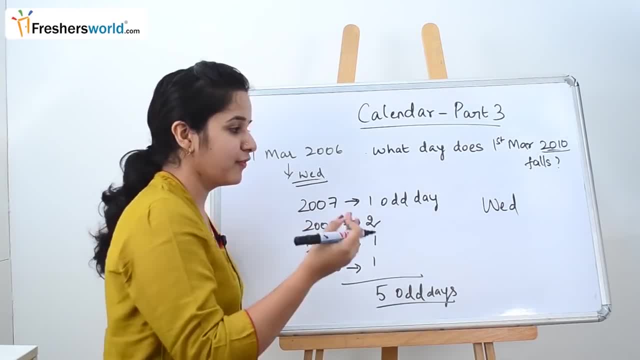 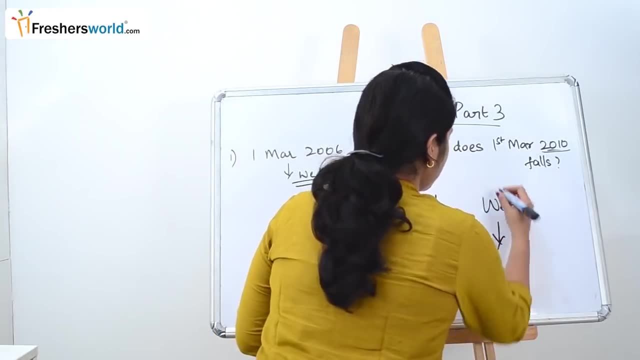 So we have 5 odd days in between. What do you do? You add 5.. So Wednesday plus 5.. So it is Thursday, Friday, Saturday, Sunday and Monday. So it is nothing but 1st March 2010. 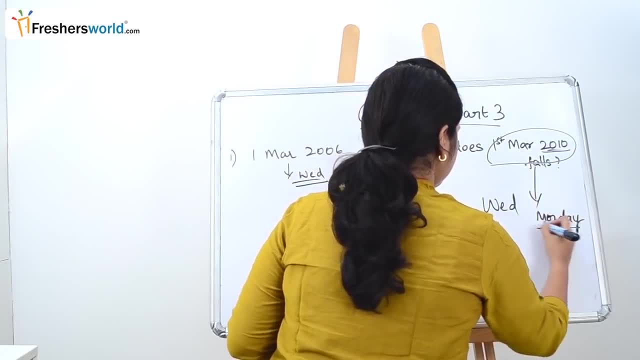 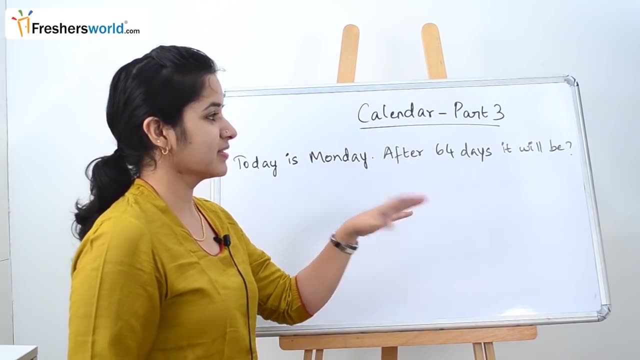 falls on Monday. Let's solve another problem. So the next question that they have given is: today is Monday, After 64 days. what is the date of Wednesday? So the question they have asked is: what is the date of Wednesday? So the question they have asked is what? 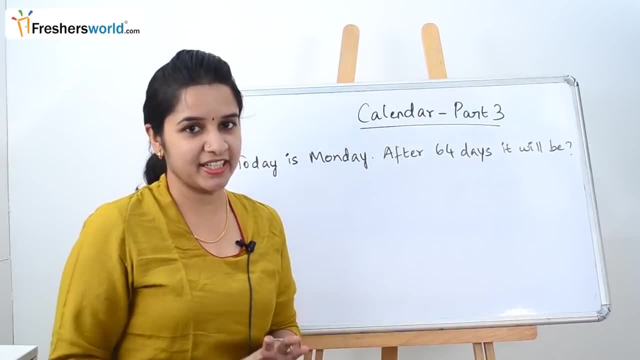 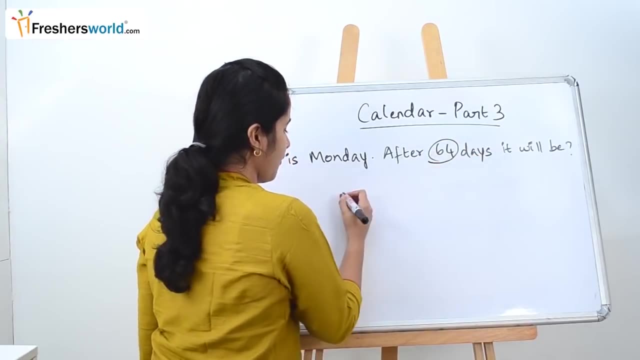 it would be So generally in a week it has 7 days, So you are going to take the multiple of 7.. So 7, take the multiple of 7, which is closer to 64. We know that 7, 9s. 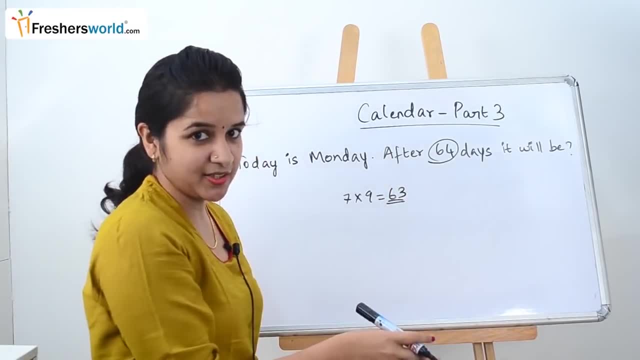 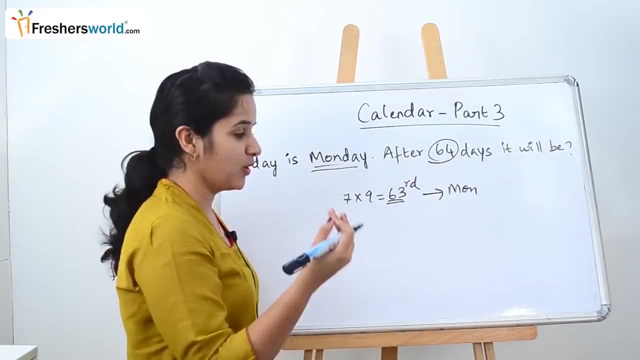 are 63. So after 63 days also, it will be on Monday. So 63rd day is nothing going to be Monday. So 64th day is nothing but 1 day added to it, which is nothing but Tuesday. 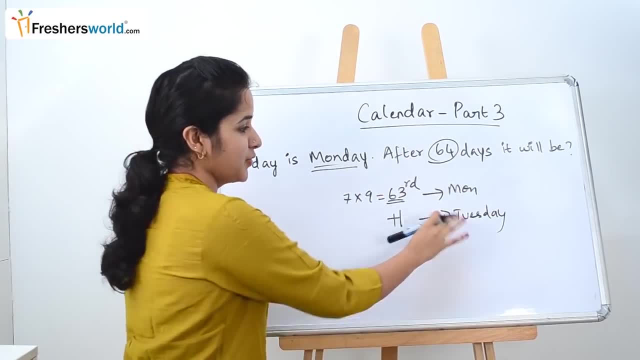 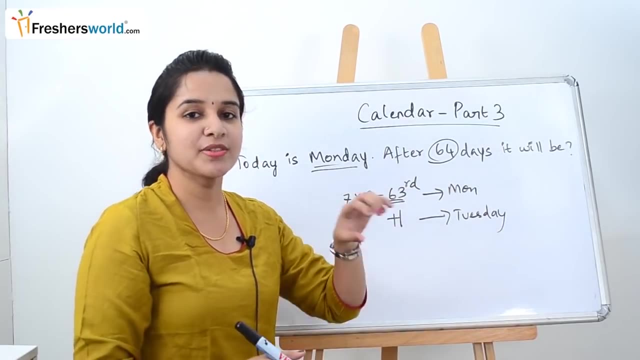 So 64th day will be nothing but Tuesday. So 64th day is nothing but Tuesday. So 64th Tuesday. so similarly, if they're going to ask you what is 62nd day, what do you do it? you know, 63rd day is Monday, so you subtract one, so 62nd day becomes. 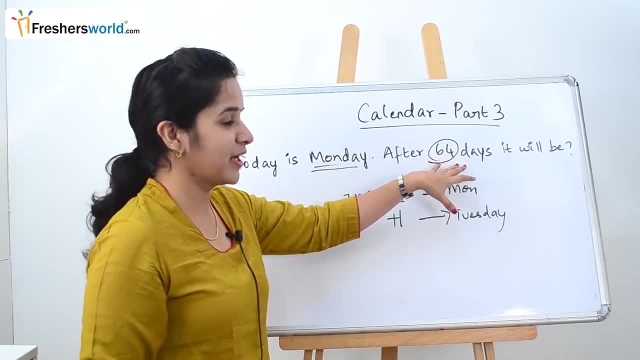 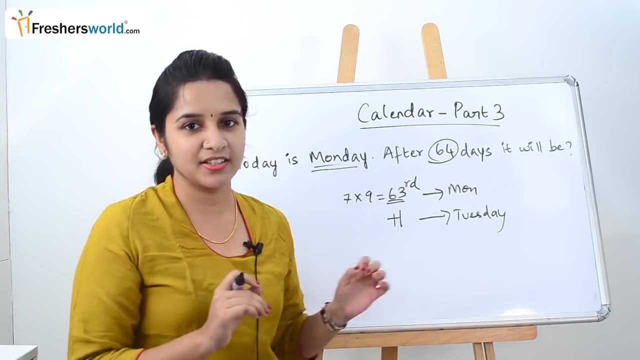 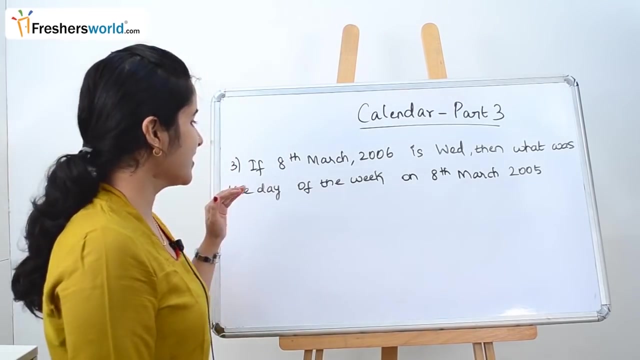 Sunday. so they will ask you the same question by manipulating here different number of days. what do you do it? so you go to the closest multiple of seven to find the correct day that they've asked for. let's just solve another some. so the next question that I've given us: if 8 March 2006 is Wednesday, then what was? 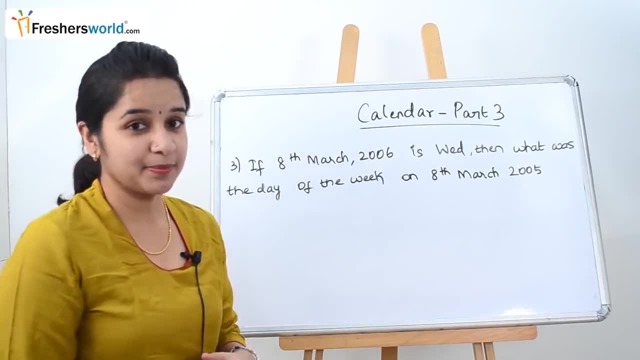 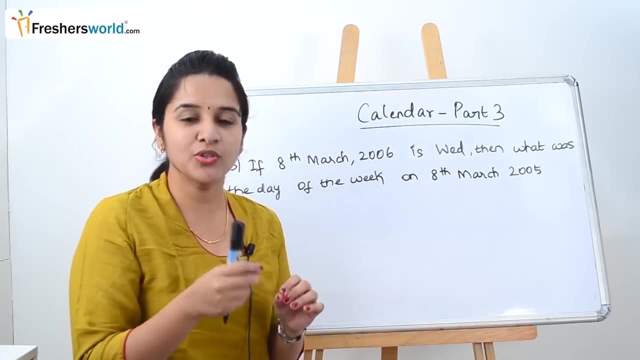 the day of the week on 8th March 2005. so it's very simple. so how do we do it? so, whatever we are doing before, there's nothing, but we just go forward. add the number of odd days. now we are going to do the same thing, but with small changes. 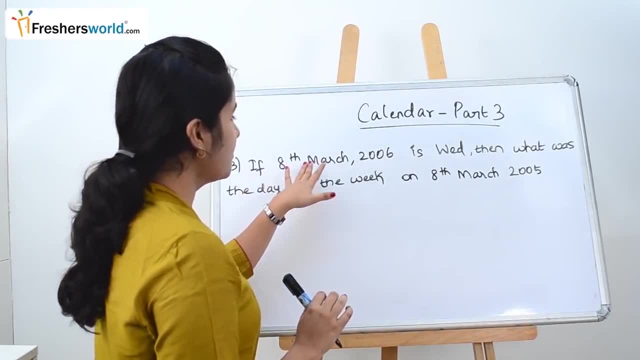 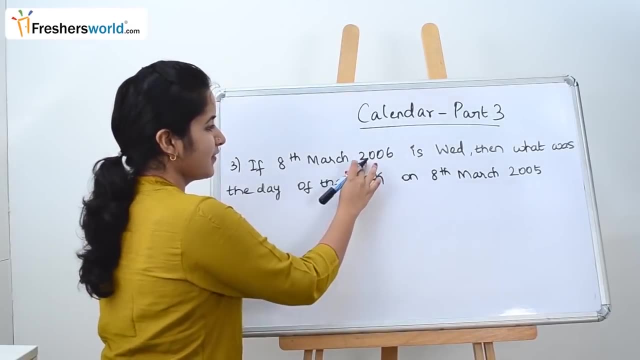 that we're going to subtract it. so here they're going to ask: if 8 March 2006 is a Wednesday, then what was the day of the week on 8th March 2005? so in 2006 we don't have to consider the odd day because we have crossed Feb there, so we 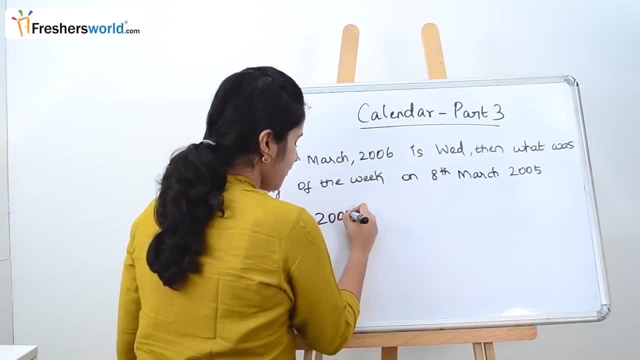 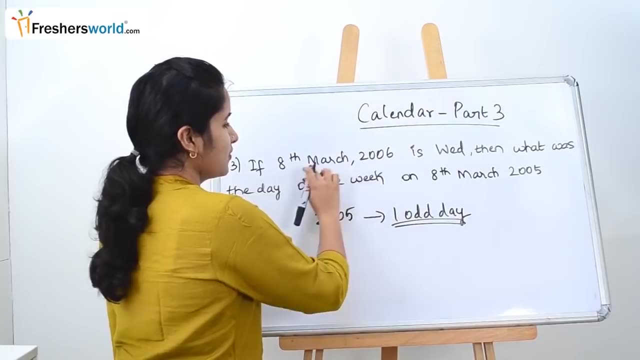 have to consider the odd day of only 2005. you know that 2005 is not a leap year, so you know that there's only one odd day. so what are you gonna do? as 2006 is a Wednesday, you're gonna subtract one day here, so in order. 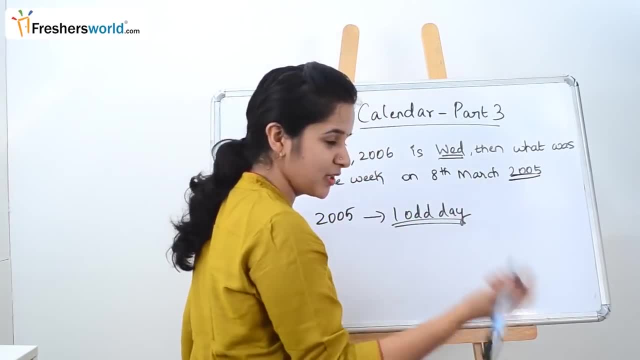 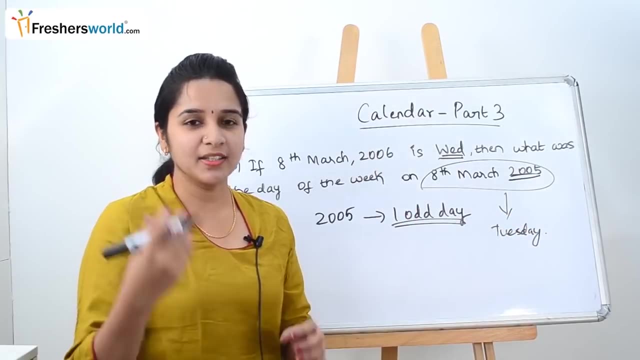 to get the 2005th day. so Wednesday minus one is nothing but Tuesday. so 8th March 2005 falls on a Tuesday. in the other problems what we did is that we calculated the number of odd days in the future, so we added it. now they have. 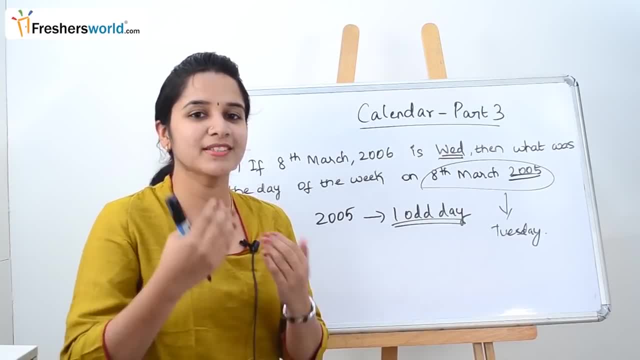 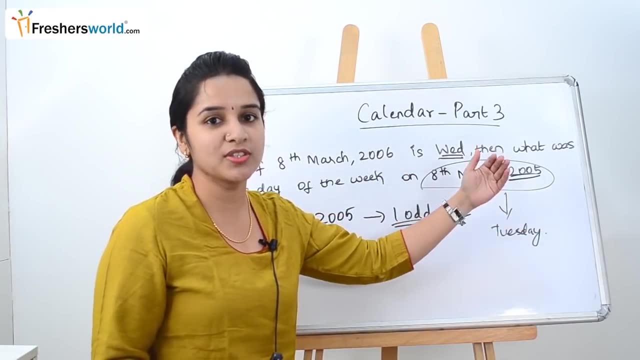 asked for days in falling on the past. so what we do here is subtracted. in the case we are subtracting one not day. sometimes they would have asked instead of 2005, they would have asked 2001 or 2003 or whatever. so you have to calculate the. 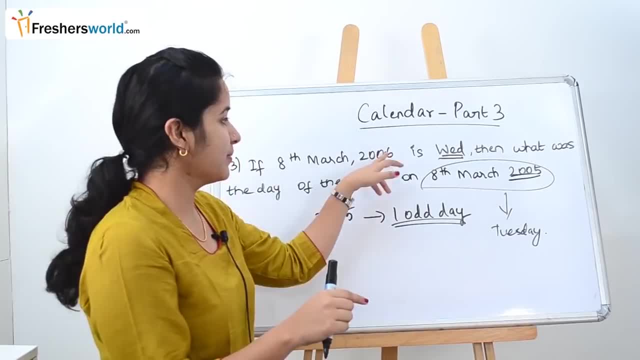 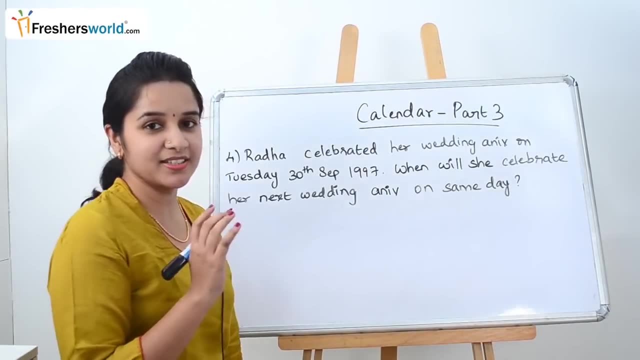 number of odd days falling on each year and subtract it here from the given day that they have given. so let's solve another of some. the next question that they've given is, rather, celebrated her wedding anniversary on Tuesday 30th September 1997, when she will celebrate her next wedding anniversary on the same. 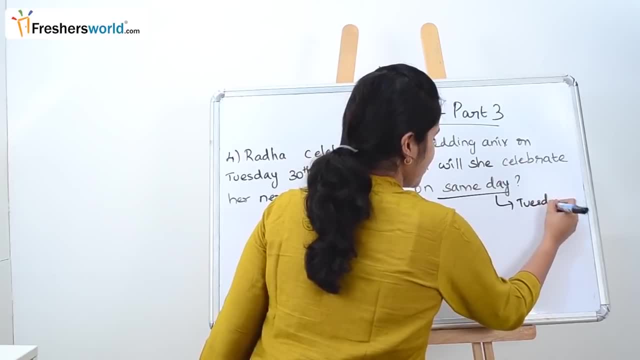 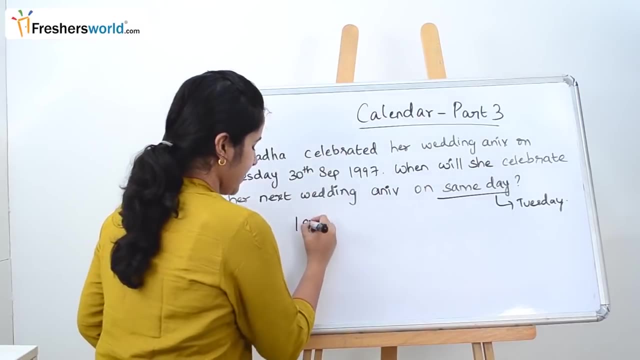 day, same day is nothing. but when they are asking again- she will celebrate it on a Tuesday- how we gonna do it? we are going to do it on the same concept of odd days. so let's start counting the number of odd days. 1998 is not a leap. year, so the number of odd days 1. 1999 is not a leap year, so number of odd days is 1. 2000 is a leap year, so the number of odd days is 2. 2001 is not a leap year, so number of odd days is 1. 2002 is nothing but. 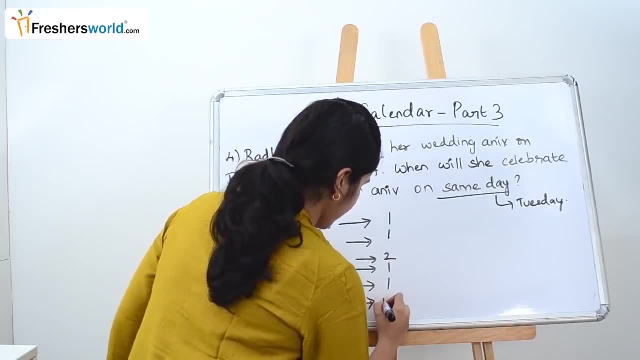 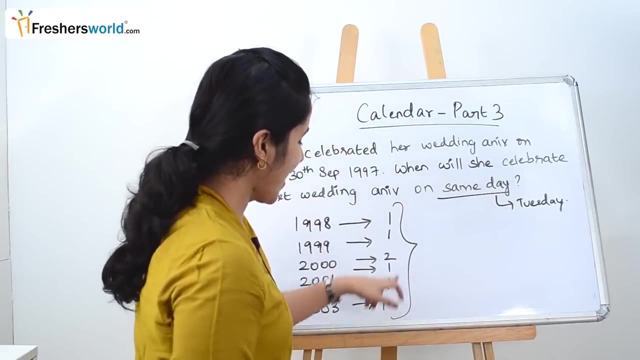 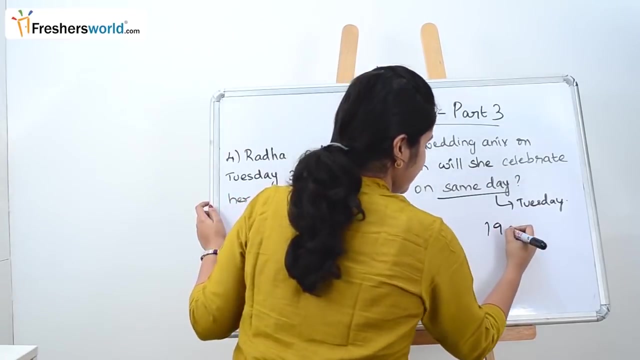 99, number of odd days is 1 and 2003 is 1. so if you add it, you will know that, see, the same day will be repeated again after every 7 thing. so if you know, if you add this, the total is nothing but 7. so this 7 comes here after 6 years, so 1997 plus. 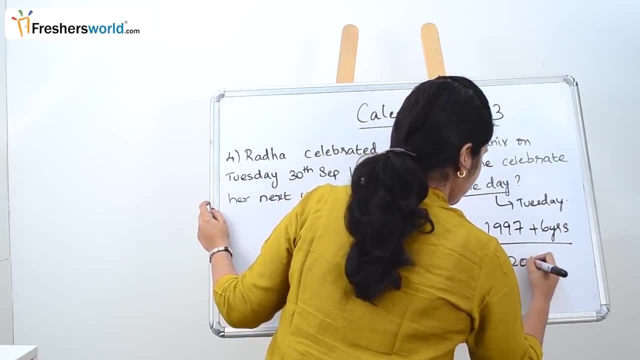 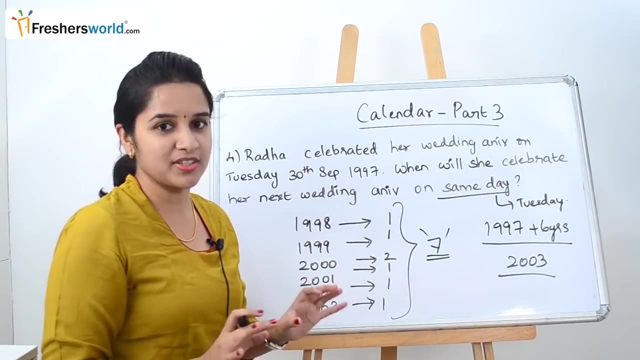 6 years. you're gonna add it here, which is nothing but 2003. so in 2003, 30th September, Radha is going to celebrate her anniversary again on a Tuesday, so this is an odd day. and she is going to celebrate her anniversary again on Tuesday, so this is. 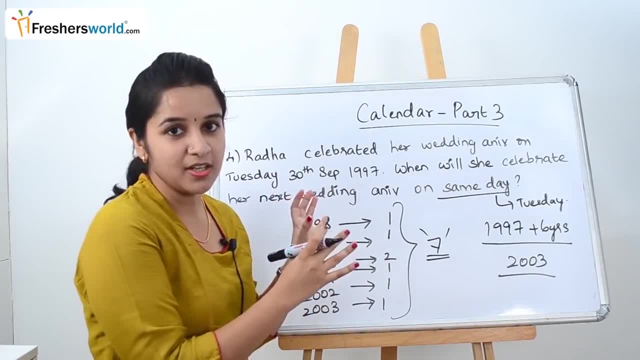 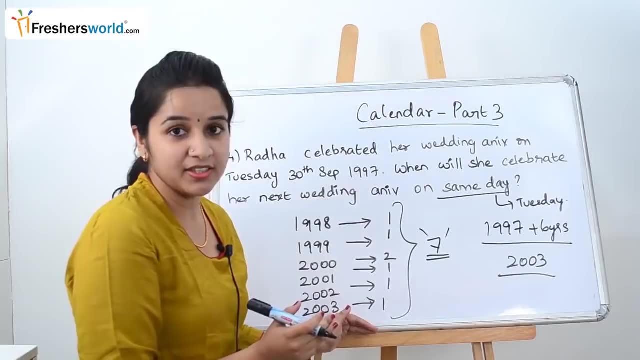 is the same way gonna follow for others, and they would have given you a different date. what are you going to do? you have to calculate the odd days. when the odd days comes to a sum of seven, then you have to calculate the number of years you have taken here and add it to get the value. here in today's video, we 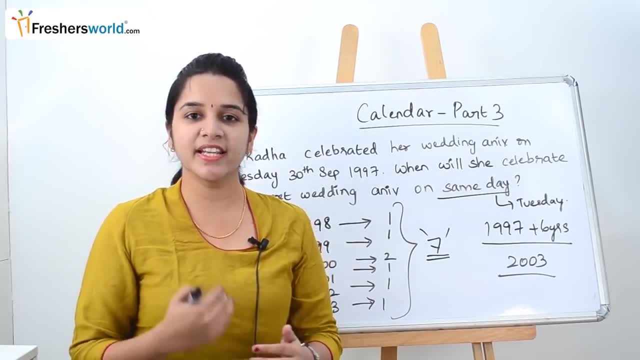 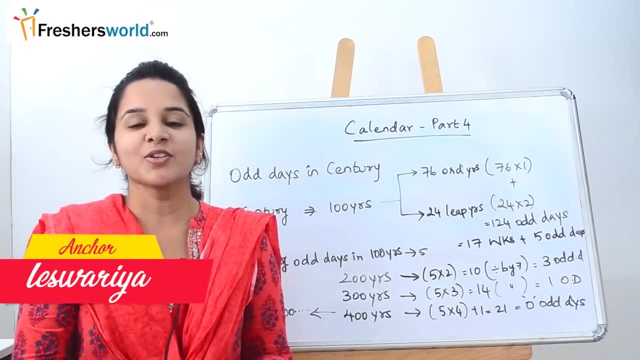 discussed about the various problems that falls under calendar. in the next video will also solve a couple of more problems which falls under the calendar topic. the topic that we are going to look today is calendar part four. so in the previous parts of calendar videos we solve various sums, so in this case 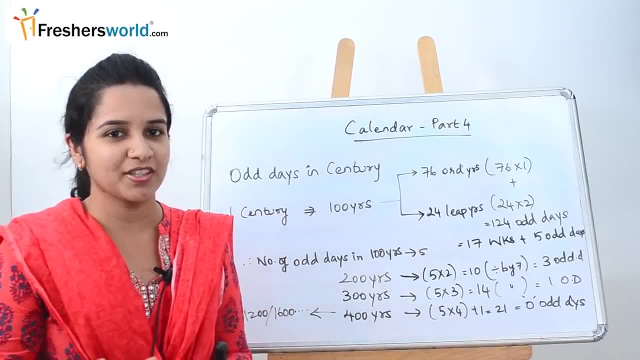 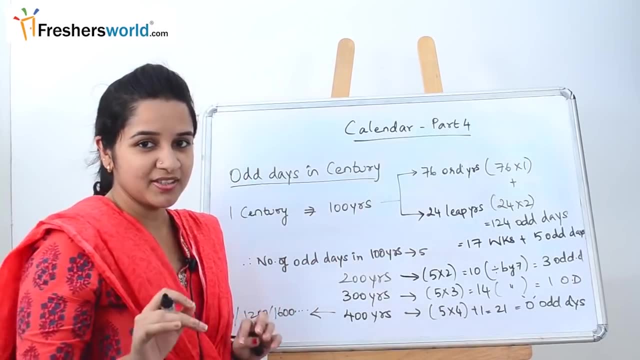 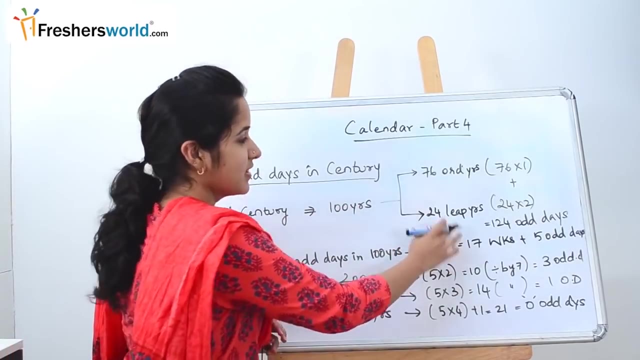 we'll be talking about the sums that are falling under the topic of century. so let's understand this concept first. so let's talk about the odd days in a century. let's take the first one century first. so one century is nothing but hundred years. so in hundred years there will be 24 leap years and 76 ordinary. 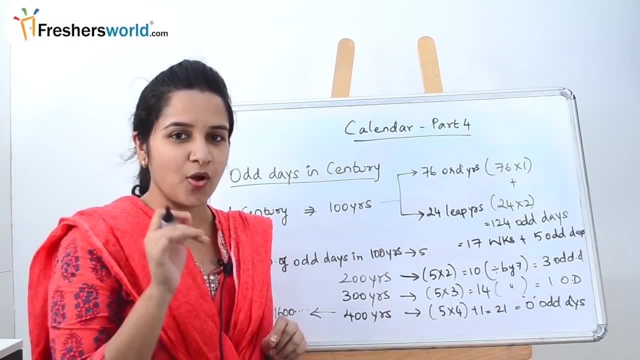 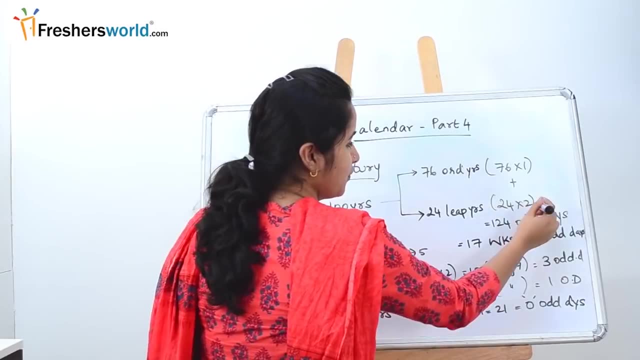 years. so we know, in a leap year there are two odd days and in an ordinary year we have one odd day. so what are we doing? we are multiplying 76 into 1 here and add it by 24 into 2, which is nothing but the two odd days. so once you multiply and add this, you will get 124 odd days. together in a single century, so 125 odd days. if you divided by 7 in the quotient, you will get 17 and plus 5 in the remainder. so this 5 is nothing but your odd days. so in the 1 century, nothing but in 100 years you will have five odd days. 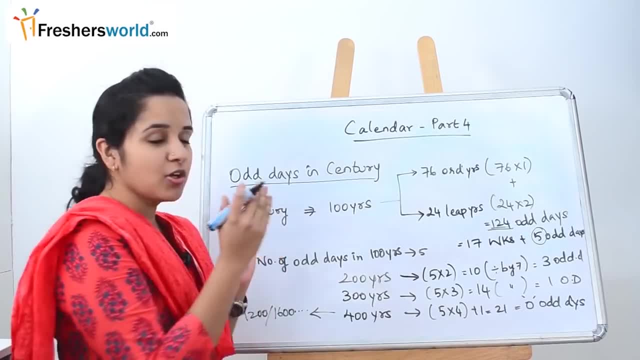 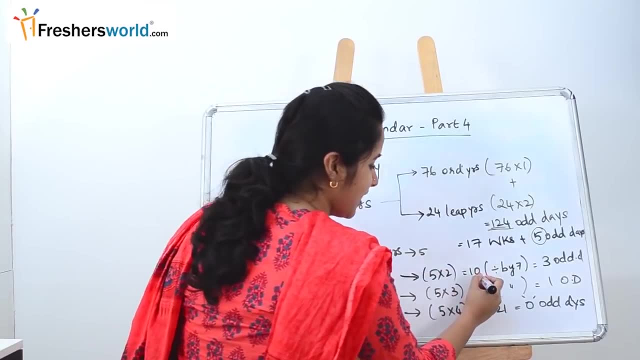 so, similarly, if you go for 200 years, this similar concept you are going to do for the 200 years, instead of going and calculating all, and what you can do is 5 odd days into 2, which is nothing but 10 odd days. So what we are going 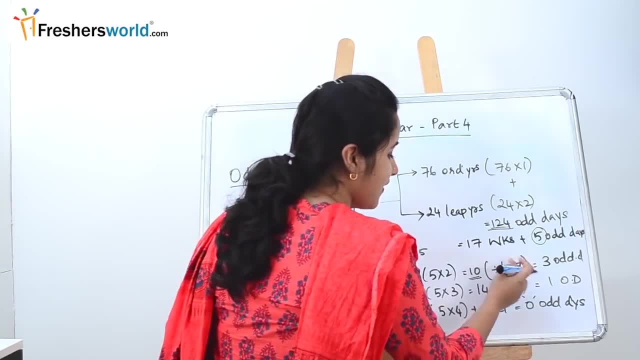 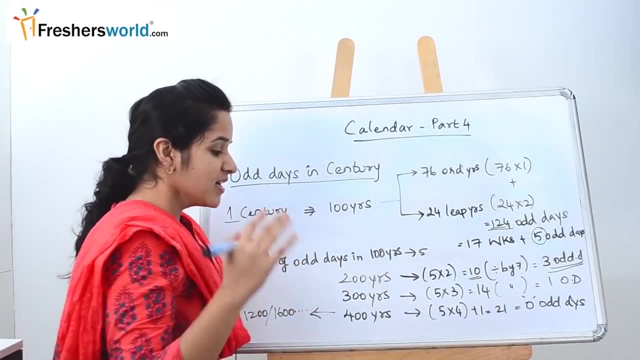 to do here now is that we can again divide it by 7.. So if you divide it by 7, we know the remainder is 3. So it becomes 3 odd days. So in 200 years we have 3 odd days. Similarly, 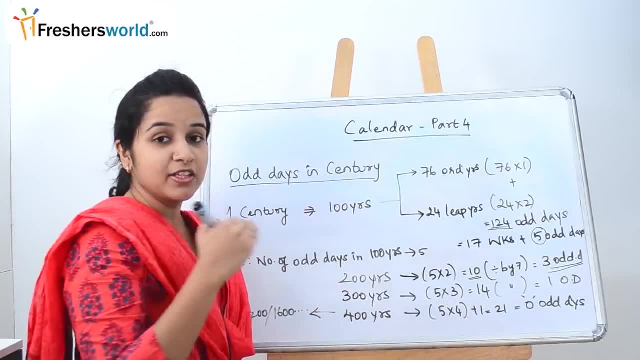 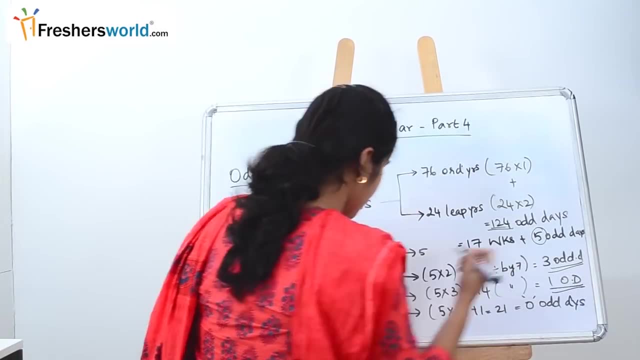 we are going to do for the 300 years. What do we do? We multiply 5 into 3, which is nothing but 15 divided by 7.. So the remainder is 1.. So in 300 years we have 1 odd day. So in case of the 400, 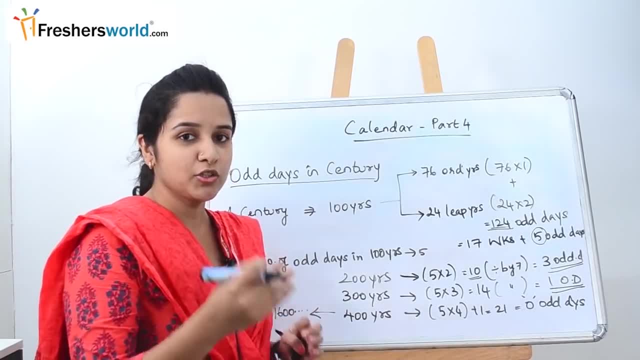 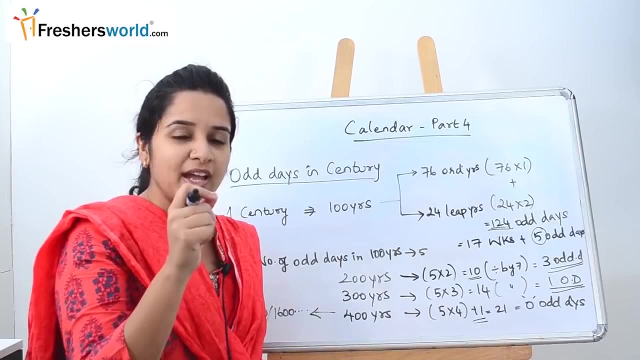 years. so as usual we multiply it by 4.. So 5 into 4.. Why is this plus 1 here? Because every 400 years that particular year will also be a leap year. So we add this extra 1 odd day, So it 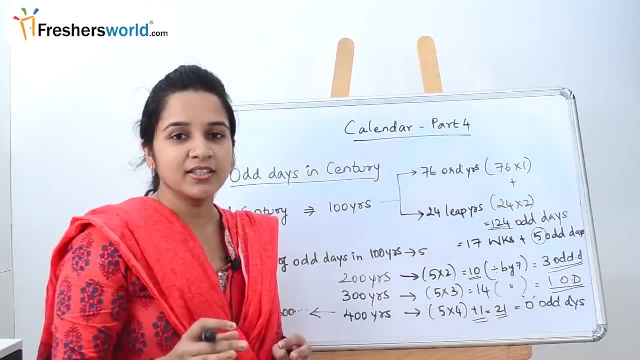 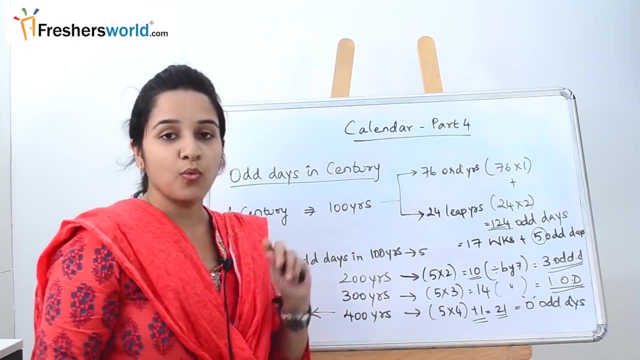 becomes 21.. So it becomes 0 odd days. So it is clear that in 100 years we have 5 odd days, In 200 years we have 3 odd days. To 300 years we have 1 odd day and in 400 years we have 0 odd. 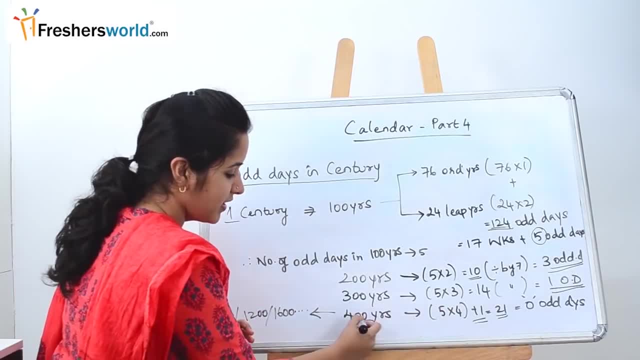 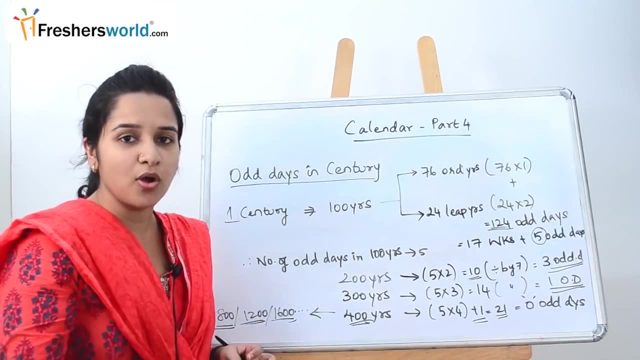 days. This whole pattern will be repeated This 400 years. 0 odd day will be repeated for the 800th year, 1200th year, 1600th and so on. For every 400 years there will always be 0 odd days. Let's solve couple of problems to understand this. 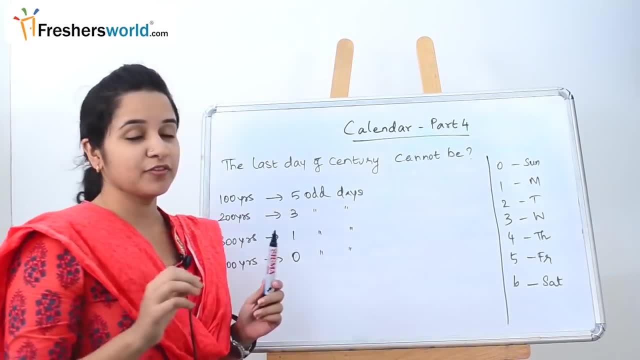 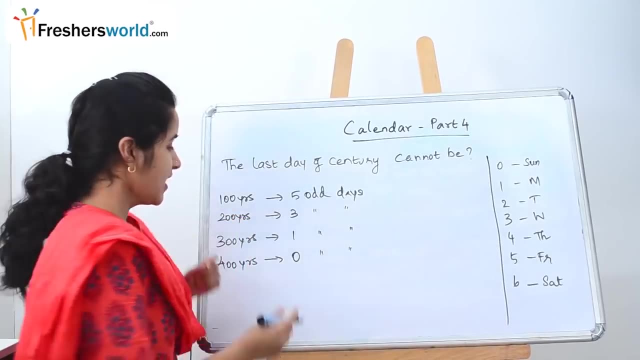 concept better. So the question that they have given is: the last day of the century cannot be So. there will be 4 options given to you. So how to solve this kind of problem. So how we start is that we know that 100 years have 5 odd days, 200 years have 3 odd days, 300 years have 1 odd.